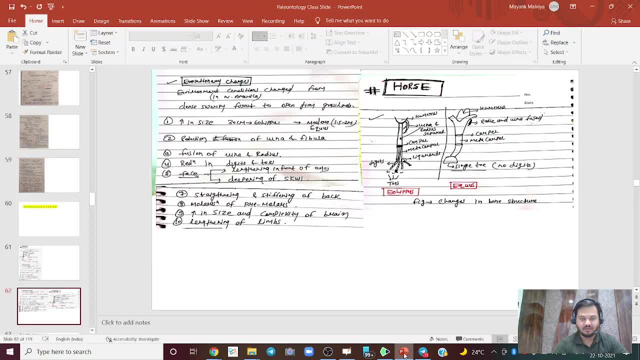 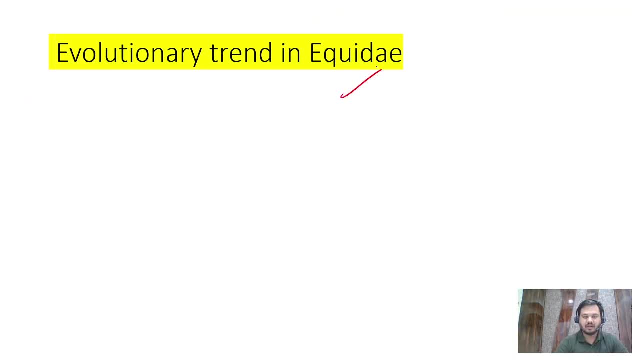 I will have to record again all this thing. Okay, I will start again. So this is our topic: evolutionary trend in Ikudai right. So Ikudai is horse only evolution of horse. and the name of horse, modern horse, is Ikwas right, The one of the earliest horse, his 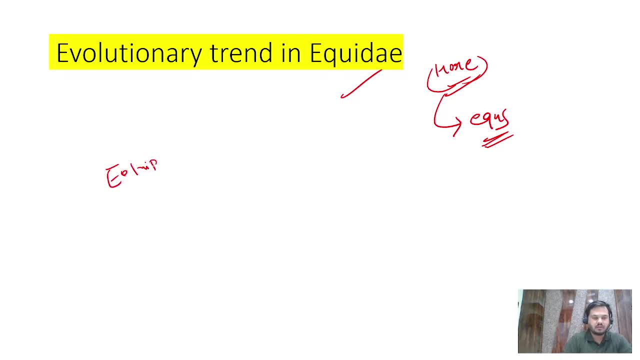 name is Yohippus right. Like if you. even if you are not from geology background, you must have sometime heard about this name: Yohippus right. So journey of horse from Yohippus to Ikwas. this is what the evolution of horse is all about. alright, There might. 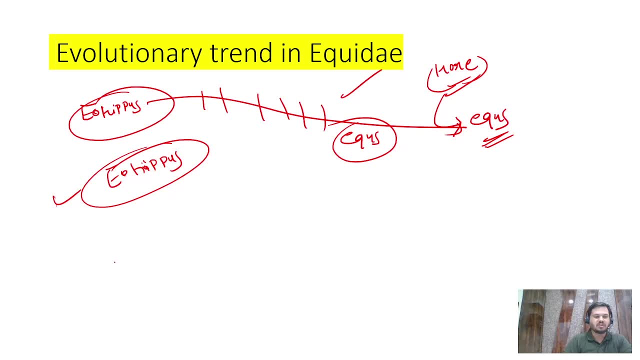 be other species, like in humans. we started from Arvoreal, Insectivorus, alright Alright Or Propelopithecus, So journey of like the species, from Propelopithecus to Homo sapiens sapiens, and then came a lot of. there was a lot of complexity, but then there came Dryopithecus. 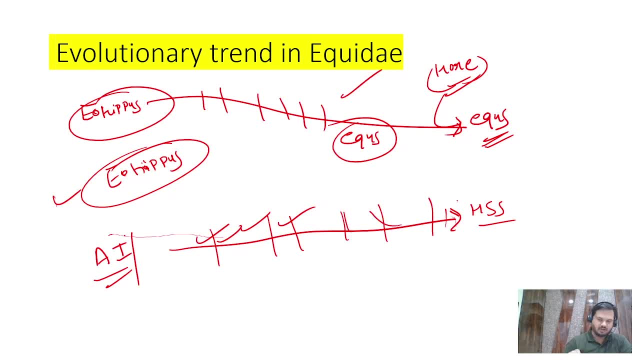 Australopithecus, Homo habilis, Homo erectus and a lot other things. Similar, similar approach is this. We will have the same approach. We will start from Yohippus. I will tell you what is Yohippus, all this thing, and then we will read few others. alright, We will. 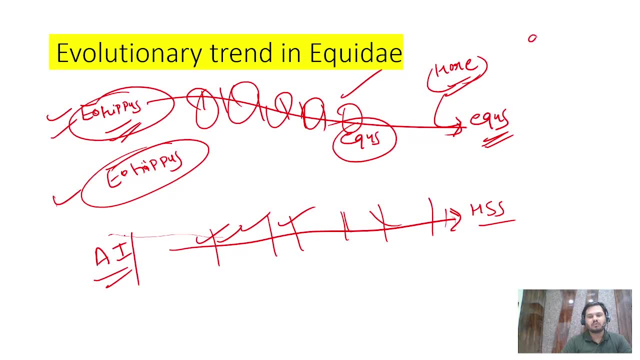 remember, You remember that there are 10-15 names and we are good to go to score at least 90% marks in this portion and we will also discuss that. you basically ask very direct question on this also. alright, So, like just to start with, we will first discuss what changes has. 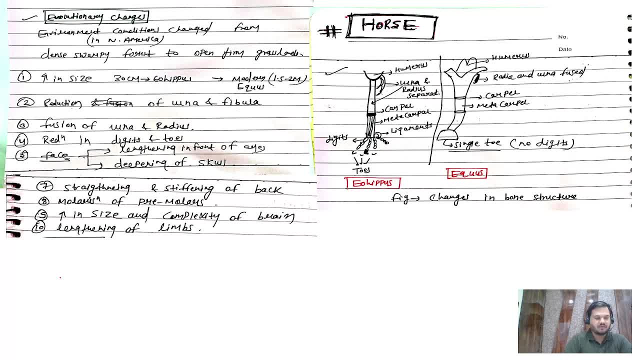 happened. right, We are not going into detail of this species. From Yohippus there was Orohipe or there was Myohippus, Plyo hippus, a lot of different species. This is also we species came up, but general what happened was like: first i was saying you this evolution of horse, modern horse. it happened in north america, all right, and due to some reason we have a very good fossil record of horse right. one of the reason is that these horses, or primitive horses, not the modern horses they lived in, hurts and maybe a natural disaster struck, maybe. 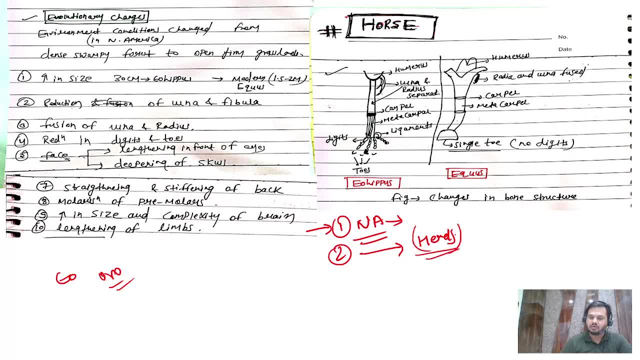 disease came, so they also died together and due to the favorable condition, their fossil was remained intact. so we have a lot of fossil of these uh animals all right, especially in the north america. so they evolved. so north america is known as cradle of equine evolution. 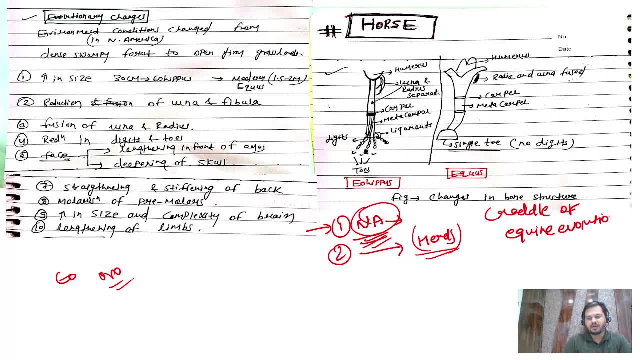 so if somebody is giving an objective geology exam, so this, this, they may ask you: north america, it is a continent, so see. so now what changes happened was. first change was there was change in environment. right so during the time of this- eohippers, it is the earliest horse, right so during. 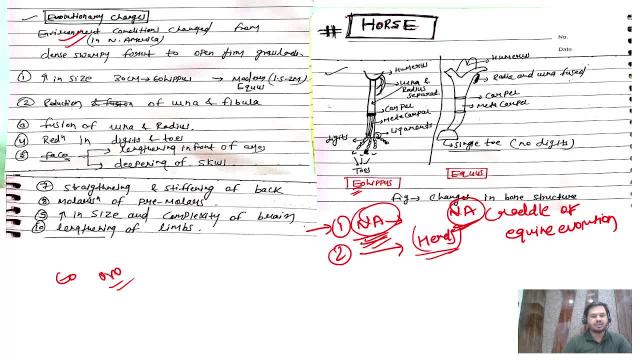 the time of eohippers, mostly in the paleo scene. you've seen time north america was a mostly a forested area, or not even a forested area, but it is. it was a dense, swampy forest, right, you understand what is swam zelda kind of. there was water also there. 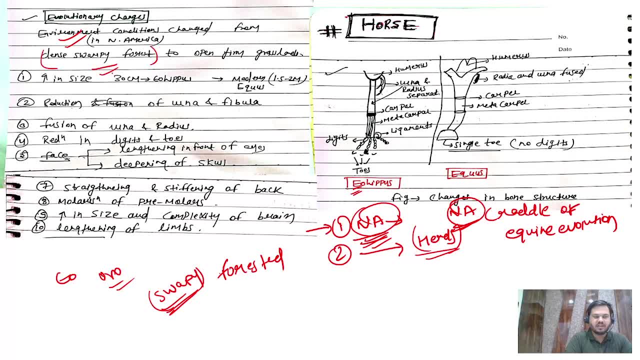 so it was a swamp, uh, dense swampy forest, and there was some climate change in that time, in, in cenozoic era, globally climate changed, all right, like we talked about. uh, we talked about the, the kt extinction, all right. so what was happening in kt extinction? kt mull of cretaceous. 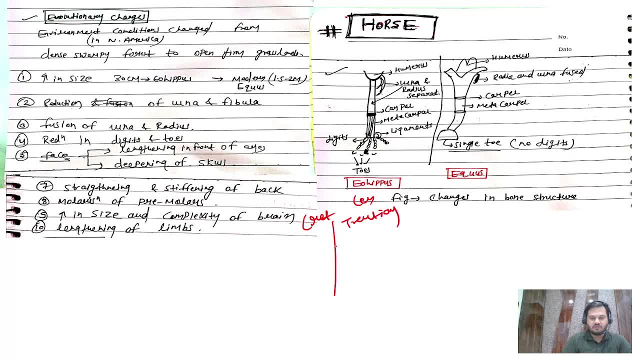 and this is cenozoic tertiary. this is tertiary time. all right. so what was happening? dinosaur was getting extinct. so what was the reason of extinction of dinosaur? like, there were a lot of reason. one of the reason we speculate is the impact of meteorite. all right, also, there was a lot. 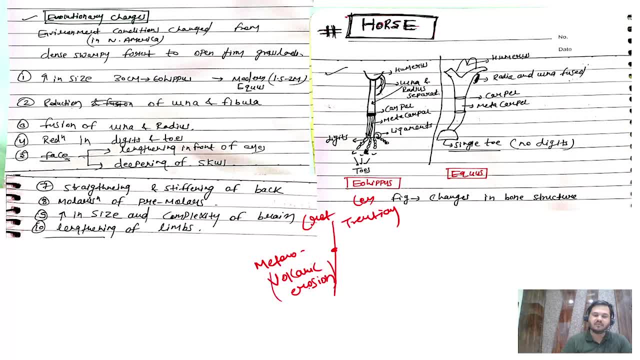 of volcanic erosion. you have seen the movie jurassic park, you could relate right. so there was also some volcanic erosion. so what? volcanic- sorry- explosion, volcanic explosion, all right. so what happens? that a lot of ash and other volcanic material was emitted and they prevented sunlight from coming to the 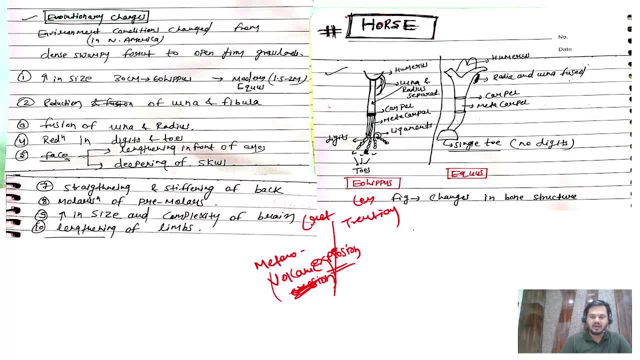 earth, all right. so there was, in general, decline in the temperature in this uniloic era, all right. and this decline in the temperature culminated in priesthood, same time. and what is like for what priesthood is famous for ice age pleasure. yes, ice ages, all right. so there was a general decline in the temperature there. 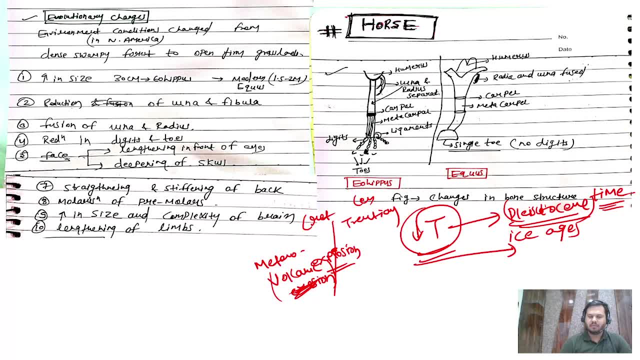 was, you know, some deflections also in between. but now, just for simplification, there was a general decline in the temperature. so these forested forests, they become, you know grassland, firm grassland, you know grassland. so this was one environmental change change happening in the north america. 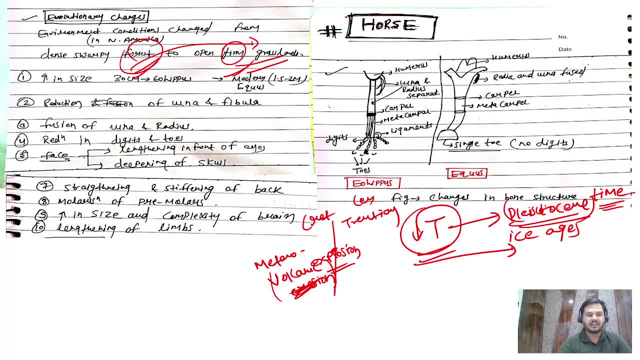 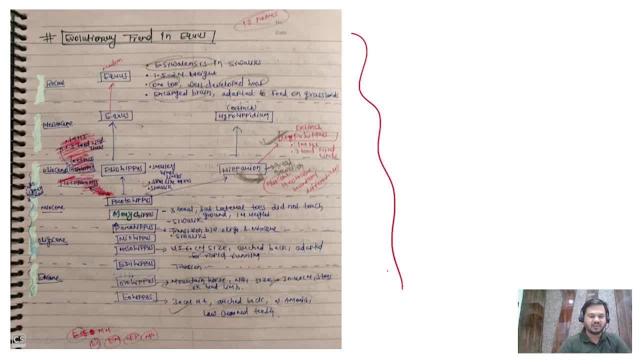 all right, so this was an environmental change. what other things happened already, like we let's discuss in the another train. so, like these are also my notes, these are also the final product. this i will share with you. so see there, the here the lineage is pretty, you know, linear. 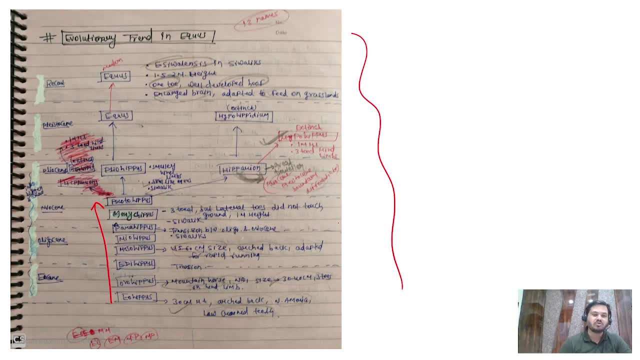 the evolution tree is pretty simple. it is not as complex as humans. so these are some names you hipers like. don't get these names, i will tell you a way to remember them, but just for your- you know- sense of comfort, i am just taking these name here. so one is, this is eohippus. now then we have orohippus. 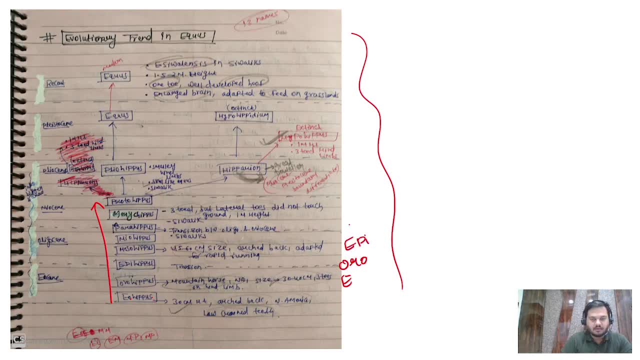 then we have epihippus: all right, mesohippus, myo para meri proto, something like this: then plio, pliocene time. what the? what horse was there? it was known as pliocene right in myocene, the whole the horse name was myohippus all right. in oligocene it was what? orohippus, something like: 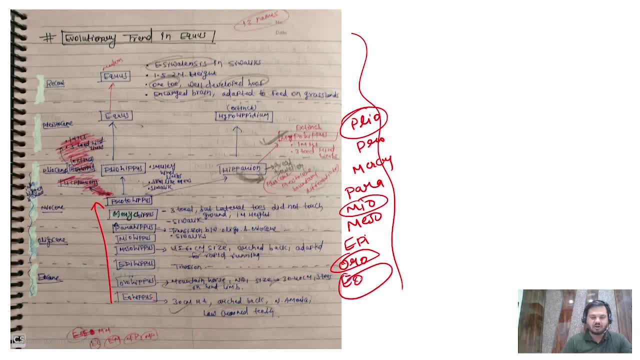 that in eocene time it was eohippus, so a lot of names are derived from the time period in which they were. they first appeared, all right. and then we have equus and then the modern equus- all right, there were some division in heparin, all these things, so don't worry, you should. 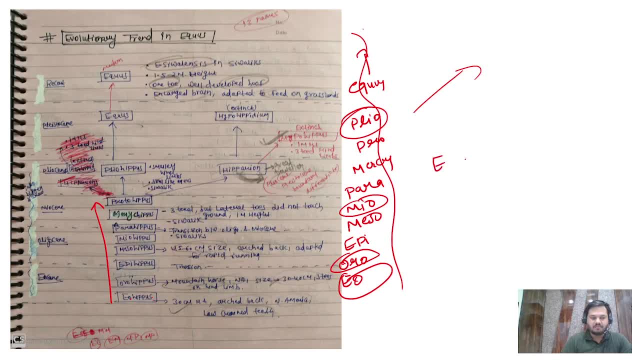 you should, you need to make your own mnemonic for it. so i, i made a very simple mnemonic: e o, e, m. i am from mp. there were two mps here, and then i know pliocene and equus, something like this: all right, i, i, i. 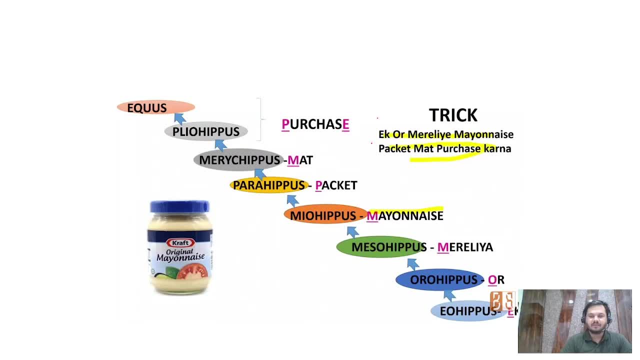 searched this on youtube, so this is not my creation. i saw a video. it was from some biology teacher and she made this trick right. so if you are from hindi background, you can use this trick right ek or mere liye mayonese packet mat purchase karna. so. 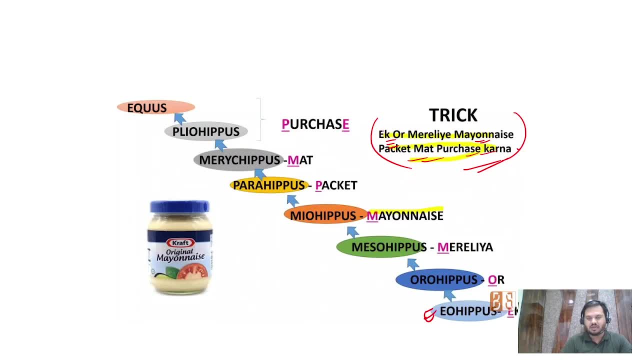 so e for my egg, for this is e, this is for orohippus, it is for mesohippus, myohippus. like parahippus, this m is for marriage, hippus, flyohippus and last, we have equals right. so, like this, like i was, i was. 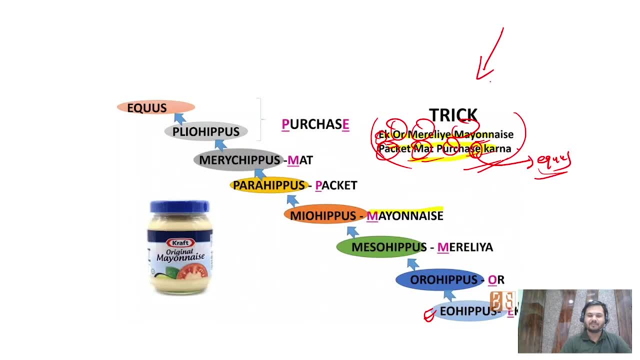 told by a lot of friend that i should not do all these things in in the class. it gives an unprofessional look, but i i don't care. i just want you all to remember these names in whatever way you can. so i am just giving you some way to remember it all right. so, like you, make your own if you can. 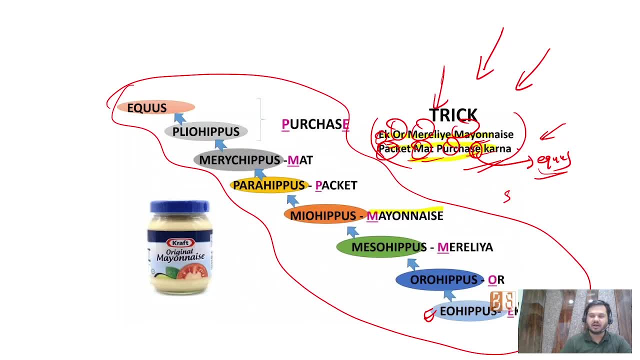 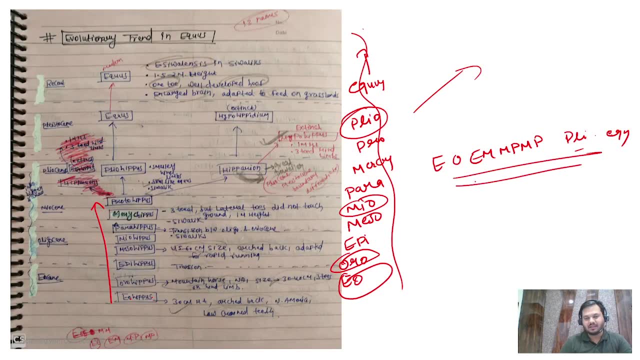 if you are from south, southern india or from, you know, northeastern india. you don't, you are not very comfortable with the hindi. you make your own one. all right, i just remember this, something like this: eo, em, mp, mp, and i could able to recall it in the exam. so my notes of my final short note for 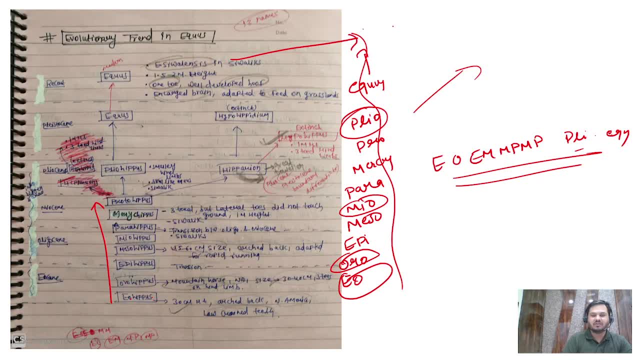 evolutionary training equals was nothing is what it was, just one liner note. and this one is what it was, just one line. all right, and i just using this line, i all, i, i like i got this question right in both ifs as well as cse. all right, and not once but thrice. so i'm pretty sure, like i, i got. 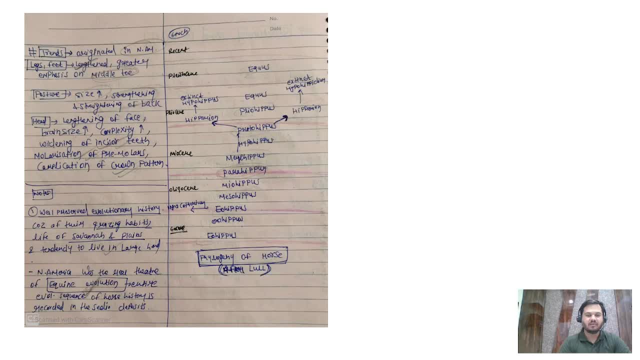 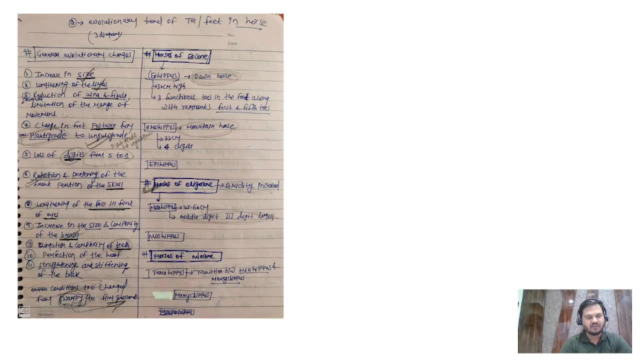 this just using this one line. so make your own mnemonic, all right, and you will get comfortable in after some minutes about this. so this we will study in the end. i think we'll. we started 15 minutes, all right, this we will discuss. so just for your basic, like understanding, we are starting this. 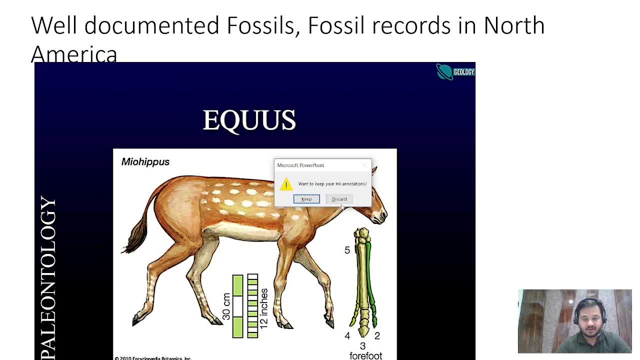 equals, right, just let me check whether recording is on or not again. all right, so see, like, just like i discussed that this is one of the most uh better documented fossil in paleontology, and uh fossil records are found extensively in north america, right, so this is some. 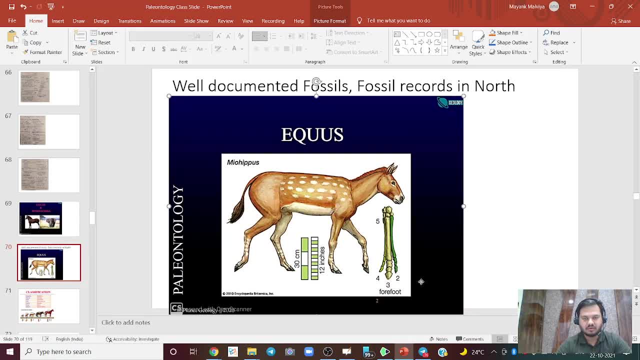 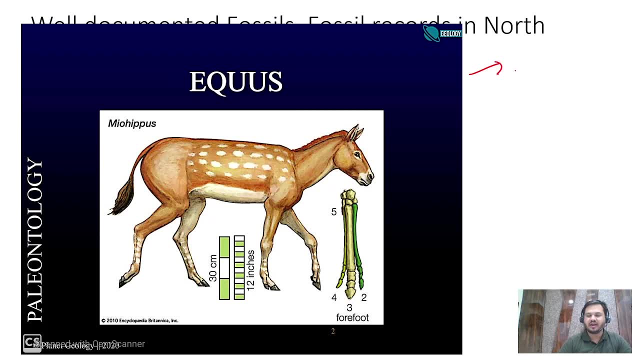 like this is just an introductory flight, like you can see. and one, one more thing about horse is that, apart from general trend, upsc, like they haven't asked yet a lot of time, but i think upsc could be like focusing next on the evolutionary trends in the foot of horse, in the foot of horse. 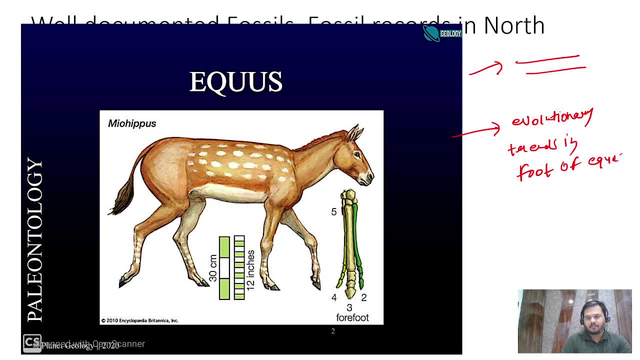 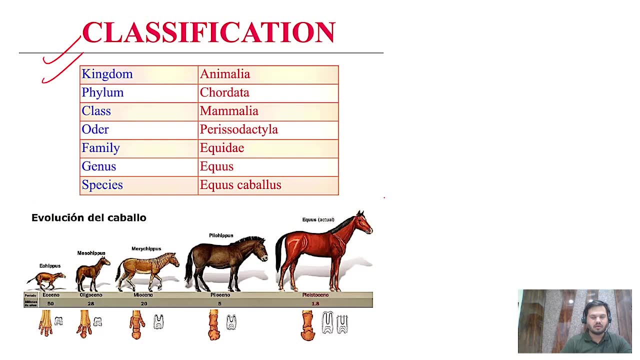 all right foot or maybe toe. so this is a very, very interesting and prominent feature in equine evolution. so this is just an introductory thing. so, uh, again, if you, you can you remember this, this could be asked in interview and you can write it in exam also. so this it could i. 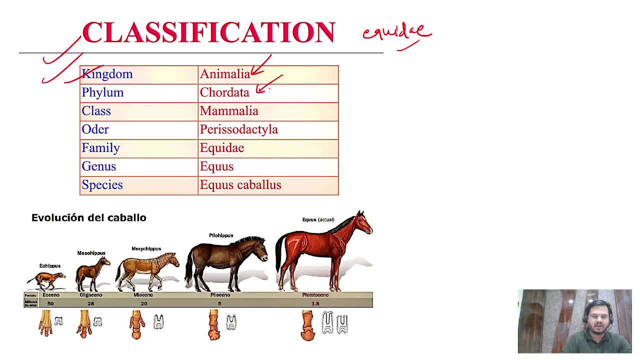 they belong to animal kingdom, just like human, chord data, phylum. they are also mammal, so this is common with human, then this is not other. it is order right, ordered. ordered is paraso dectila. all right if you, if possible, remember it. you can even ignore it if you are not very comfortable, but remember this: these are. 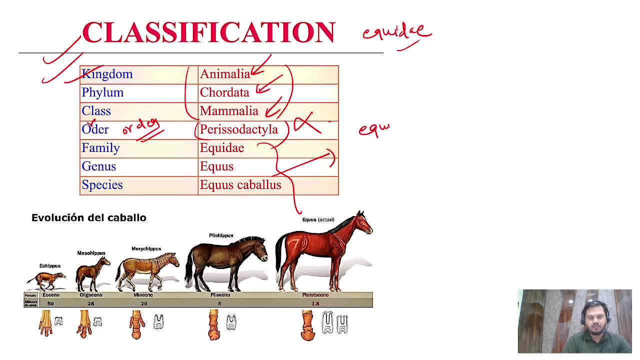 very easy. so they are from ecudae. family ups has mentioned, as the family itself, school family equals genus and equal species. right, they are equal species only. so this is a general trend. right now, you people, like you did with humans, you tell me what general thing could you observe in this trend? right, this is the earliest horse quote. 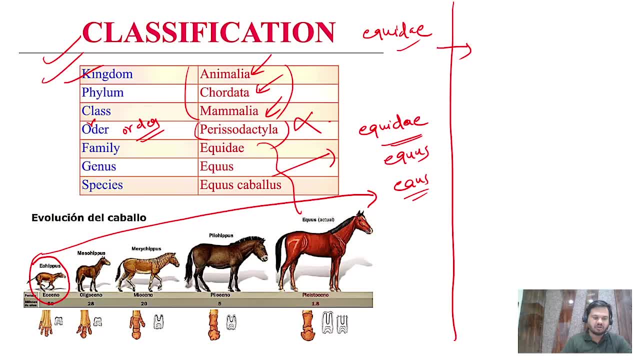 unquote: horse, the most ancient ancestor of horse, which we call as Eohippus. then there are some other names, ignore it, Mesomerci, whatever, but you can actually see the diagram. tell me what are the things you could observe in this diagram, anyone? how it is increasing. very good, what else? getting hairy, sure? okay, I don't know. 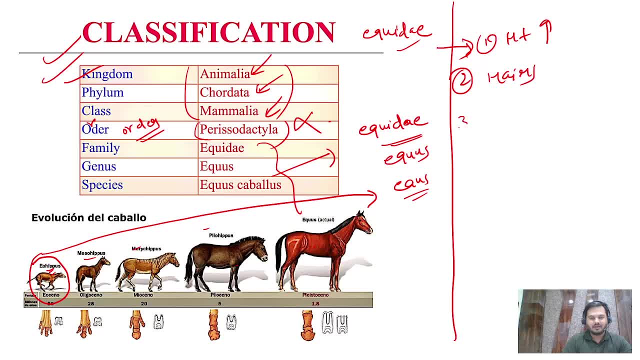 what? okay, you are you like something related to here's all right, and you can see, sorry, foot of the horse leg, something like. I cannot, it is not audible, but I think something related to foot. so I think if the length of the legs are increasing, all right, you can also see there is also an increase in this, this size, all right. 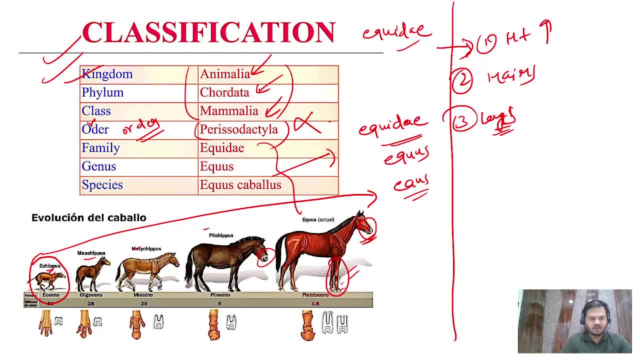 this size, right, what else you can see? so muscular, it is becoming more muscular. it would also be increasing. this is a normal evolution, all right, but in capacity must be increasing. but also, you cannot see the foot, but like I have used this small image here, there is a change in the foot also right earlier even they. 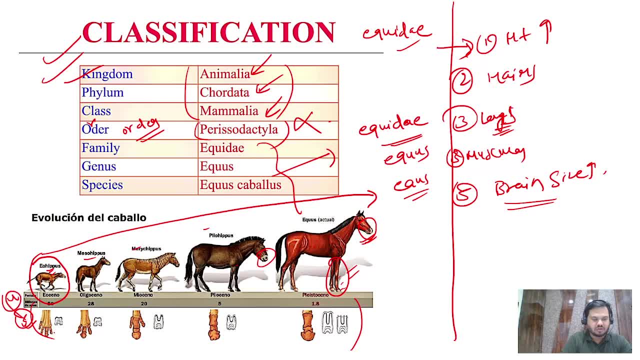 had 5, two, all right. some speeches are 4 to 5 toads. you can see here, alright. then they become 3 towed, then after that I can see this creature and more… 3- Meow or 4-5. One is there in the water. why is I told by someone? then they become three toad, that they are normal evolution. all right, so I see that. so makes it clear. it is saying that if you have a base, I just wonder how to understand all of this interaction. I am going to keep this for you now, NaBeanFR. 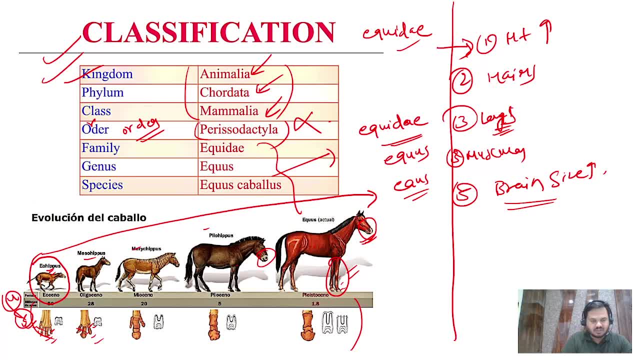 institute also takes connect with you. let me show you palm toad from elsewhere the guy is now. Then what happens is that the digits of the toe, you can see they are becoming smaller, and this is the bigger one, So this might not even be touching the ground. Alright, And then all these fingers got disappeared. We get only a single toed horse, and the modern horse is also a single toed. 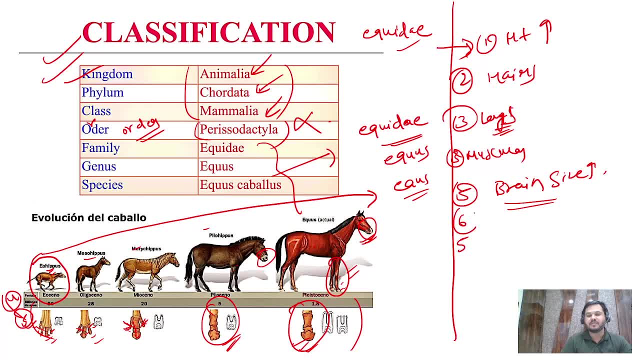 So you can see it was. it is the most important feature. It was a five toed animal to. it has become one toed. One thing is also: there is a development of hoof. Alright, Like when I was reading this book, I didn't have much interest in wildlife. It was like years ago, Right. So I didn't even know what is hoof And I was very, very, you know, shy to ask you what is the meaning of hoof. 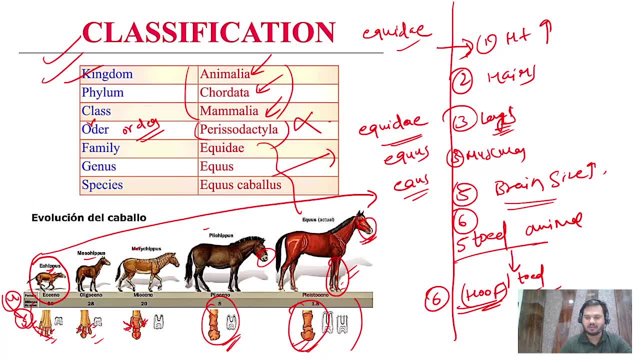 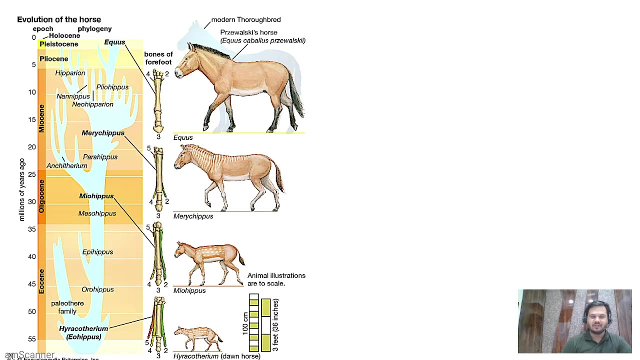 Okay, Because everybody sitting around me in the college they know what is hoof. I was even confused. What is the difference between toe and fingers? Alright, And why you are taking the names like digits. So like, if you have such doubts, like, feel free, you are, you are learning from a guy who also learn all these things on his own Right. So, don't worry, I have included all these things in the slide itself, like for your understanding. So like this is: don't worry, we'll come to that thing in few minutes. 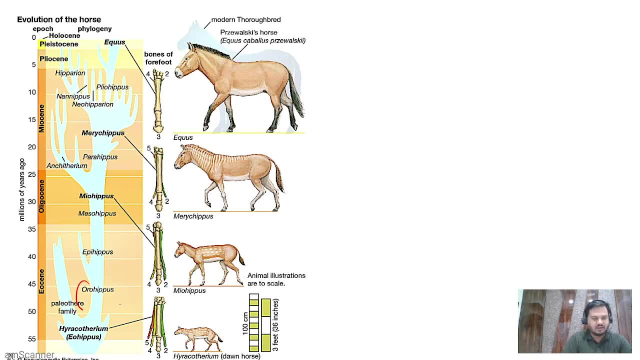 Right. So this is a general evolution. So, like I said, you know this, Oro hippos, Epi hippos, Meso hippos, Mayo, hippos, Mayo, hippos is alright. Then there is Pera Massey, all these things. So this is a general evolution. One change is, one trend is see this: This is nothing but the lag, Right, So it was from four to, or maybe five toed to, they become three, they become then two, one and four, they become extinct. three become more prominent And then presently, in equals, we have a single toe, one. 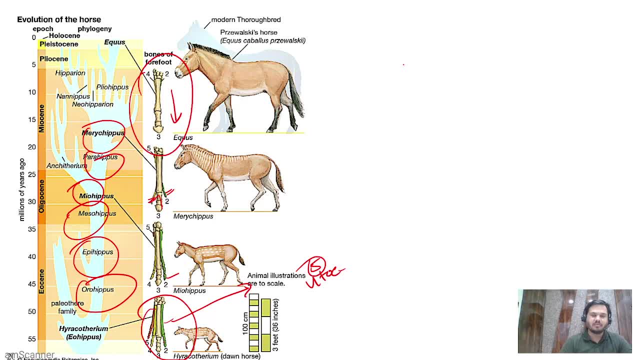 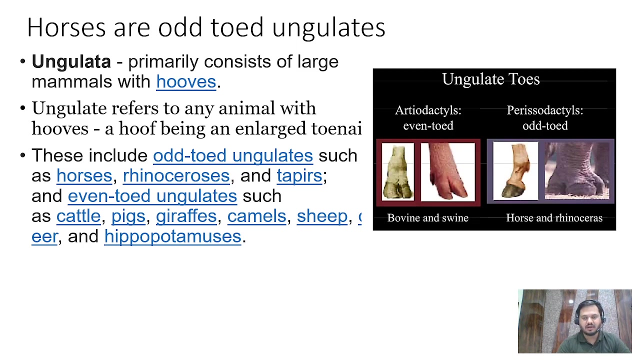 So if anyone, if you like, today we live in a modern society, we are not much, we don't have much interface with the horse, But maybe if you are from a school which has horse riding or you are lucky enough to see the hoof leg of the horse, you can understand this pretty easily. So don't worry, I have included few slides, Alright, about the horse. you will see there. So presently, the only interface with horse is during marriages, Right? 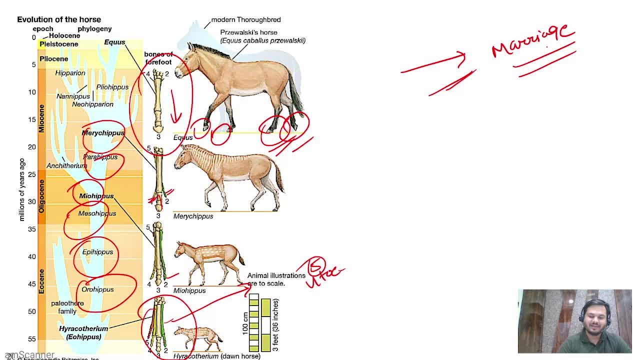 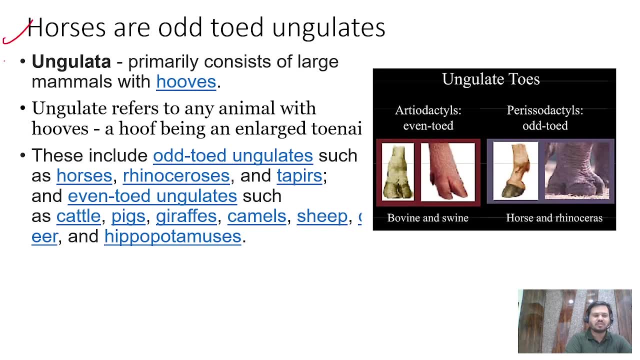 The groom sits on it, That's it, And we don't have much interface with this beautiful animal Right So like. this is a very common line written in the book- This is not very important from geology point of view, But still I've used it- that Wikipedia says that horses are odd toed ungulates. Alright, So I hope you know what is the meaning of odd. This is even an odd. So one, three, five, six, seven, eight, nine, ten. 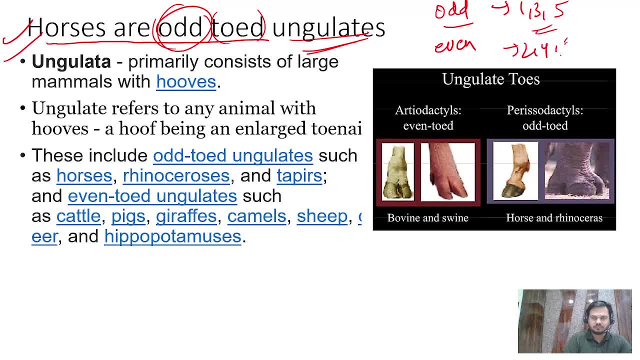 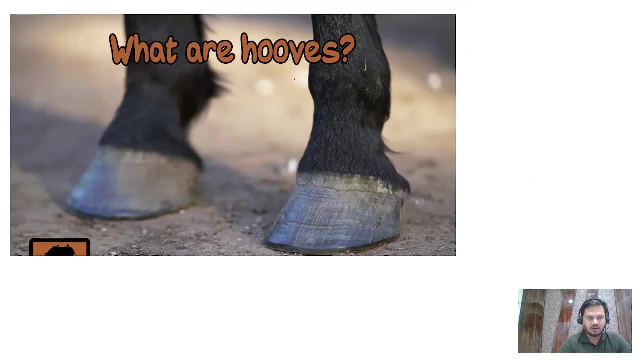 Five, something like this, Even it's two, four, six, something like this. So they have odd number of toes. So horses must be having one, three, five kind of like. presently the modern horse have one toe only, So they are odd toed. And ungulate is some animal which have hoof, Alright Or hoof. So what is hoop Hoof? is this? You must have seen even cattle. If you have seen cow, you must have seen cow. 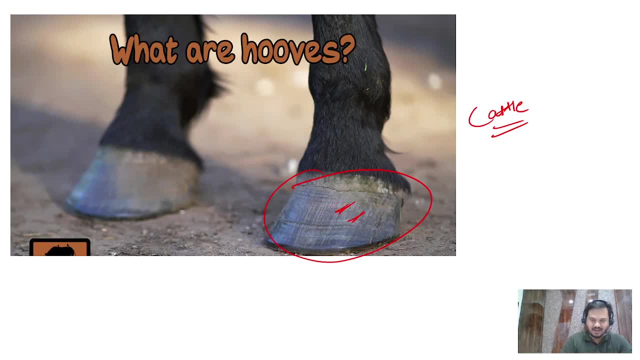 Even it has such hooves, Alright. So this is basically nail kind of a thing, Alright, This is just a single toe And this you can see, even like have learn it like this is nothing but a nail kind of a thing, Right? So I hope now you understand what is hoop. It's like tip of the toe, Yes, Perfect, Perfect. It is actually tip of the toe, Sorry, Tip of the toe, Right, Just like we have this nail. 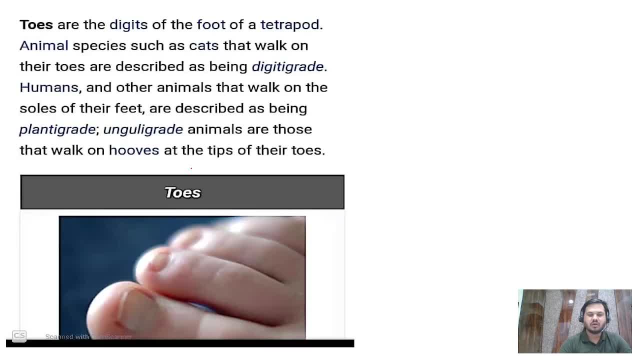 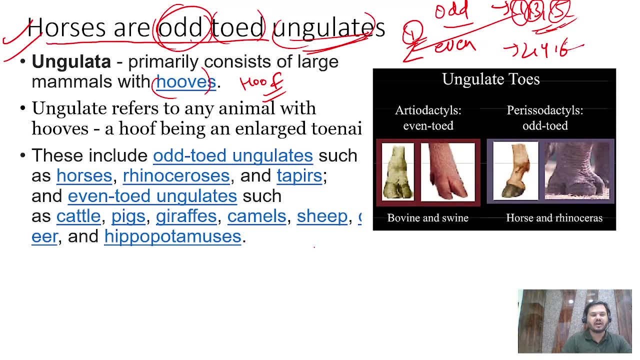 So surface of the nail, that is something like this. This is hoop, So this developed in them. Alright, So, like there are, animals can be classified on the basis of number of toes, Alright. So ungulate refers to an animal which have hoof, So it could be in a rhinoceros have hoof. horse have hoof, even cattle, pig, hippos, camel, all these have hoof. So these are ungulates, different kind of ungulates. So don't you don't have to go in detail And you can see this is bovine cow and all They have hoof. 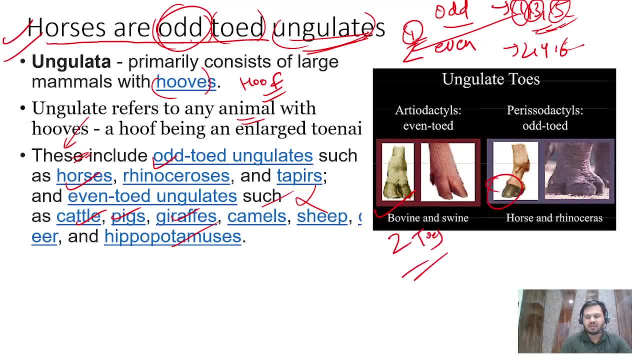 Two toes. This is horse It has. even it has a single toe. Rhinos have generally three toes, Horse has one. So this is just for your understanding, Not important for exam point of view, But like: if you are smart enough, you can. if you understand all this, you can chapeau this line In exam. horses are odd toed ungulates, without getting bothered about the terminology, Right. 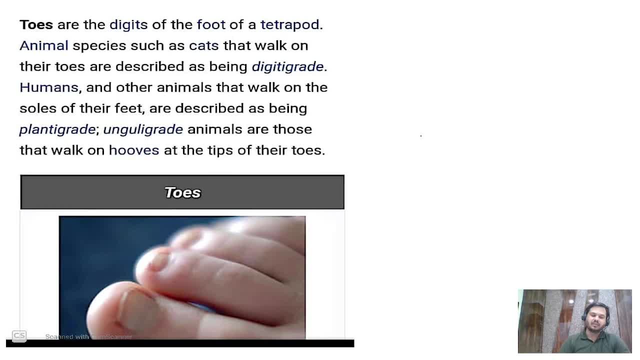 So this is it. Now, just somebody like I took this class in one of the crash course And a guy was like very shy to ask me the difference between toe and finger and all these things. He was getting confused on on these terminology itself- So just if maybe some might- someone might be here also- is confusing, Like these are more or less the same thing: Finger, we talk. we talk about finger in terms of our hands, right, All these digits of our hands, apart from the thumb, we call them fingers. 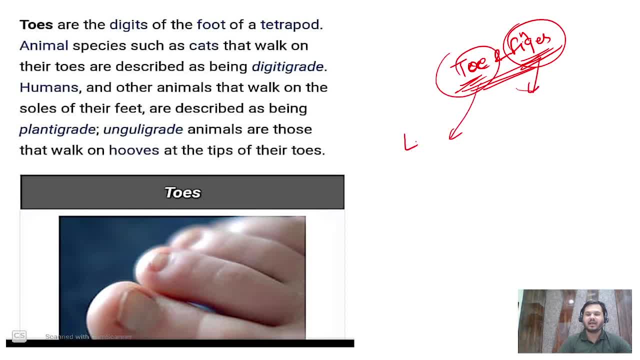 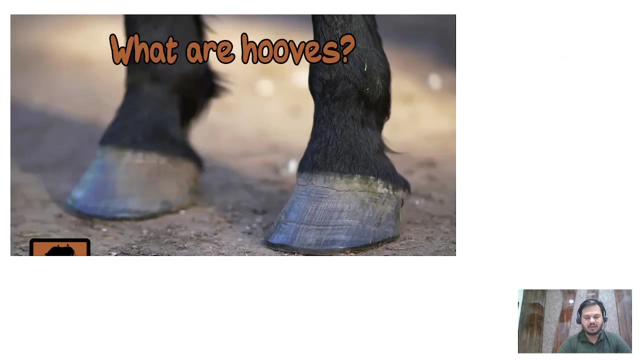 Right. Similarly, the digits of our legs. we call them toes. So horse don't have hands. In a sense, all its limbs could be classified as legs. So we talk about toe there. All right, So, like, based on this, toe, toes are the digits of the foot of a tetrapod. All right, So something like this. you don't have to go in detail of this, Right? I just use it for doubt purpose, Right? So I've also written here the difference between toe and finger. 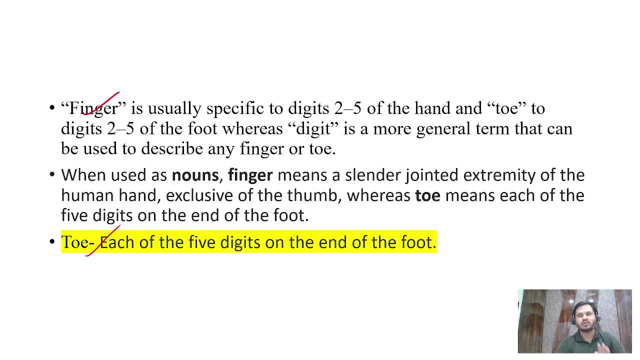 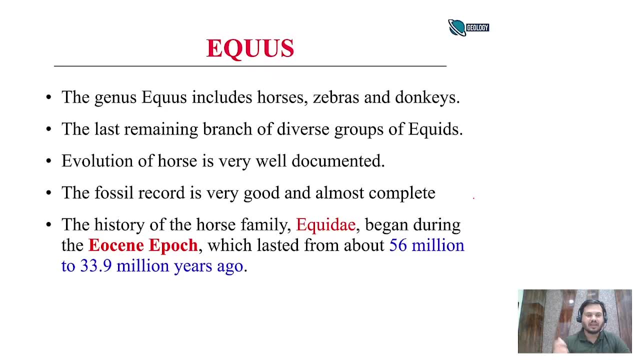 Toe and finger, if you want to read, but I hope like it is fingers related to hand. toe is related to the foot, Right, So we talk about toe in all this. So, like equals, equals is a genus, All right. This include horse, zebras, donkeys, all these things, Right, So see, and the best part is the history of horse. It originated, like it began, around 50 million years ago. Just remember this fact. I don't do don't have to go on all this, This equal. 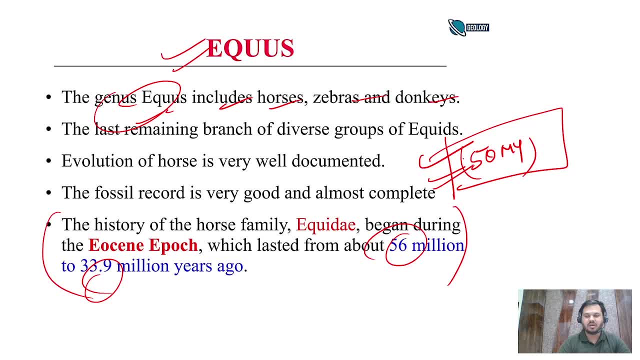 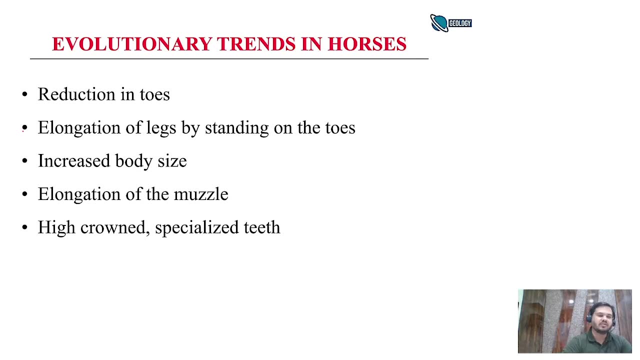 Because the history of equals evolution. it started about 50 million years ago, So 50 million years ago is some somewhere around Oligocene, I think. All right, Paleocene, Oligocene, boundary Right. So what changes happened? What are the evolutionary? This is the last slide And specifically we will study tomorrow. So what are the changes happened in the horses Right? So I want to show you a picture. 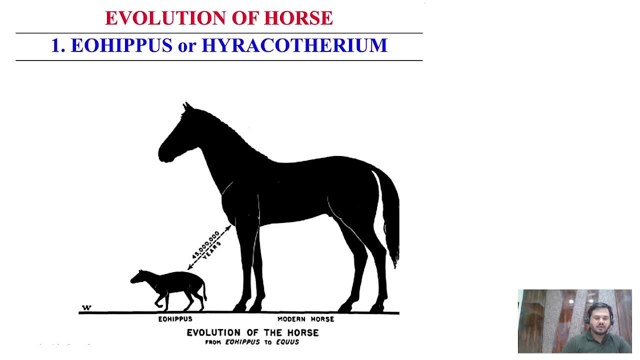 This, This. So this is what this is. your hippas now a pins ruled was. I have taken this name. I have taken this name for five times. You, hippie, At least you should be comfortable with this name, and this is modern horse. 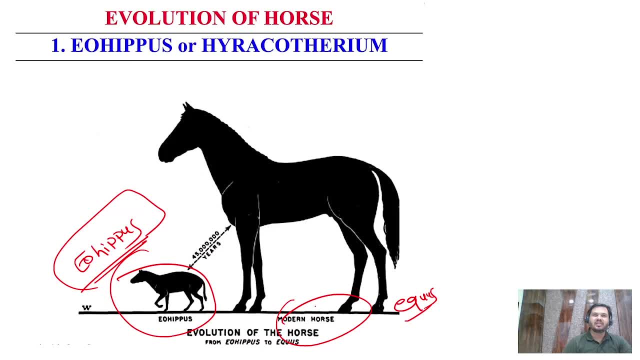 If you put both there, both of them, in a picture, This is what they will look like, right? So the history of evolution of horses is history or this History, or is just that History? or is just that History, or is just that? 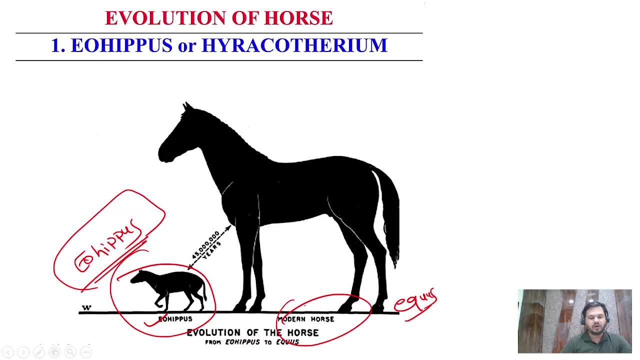 History, History, or is just that History or is just that? journey from hip us, you hip us, to modern horn, all right, so like what changes have happened? you already have top and see its size has increased, right, weight has increased. obviously, size will increase, weight will increase. all right, then you can see that here. the back. 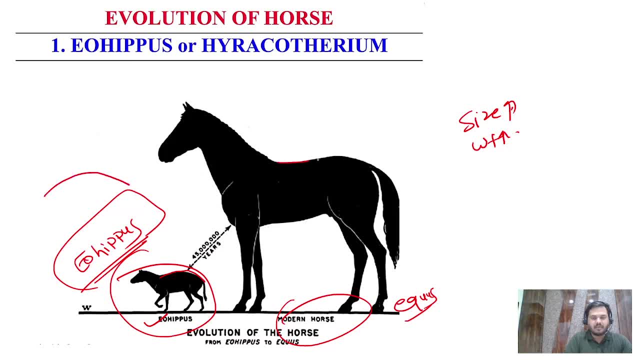 is a bit bit curvy, linear right, and here the back is more linear, all right, and it, the back, has all the stiffened. why it is stiffened? because humans started sitting on them, all right. human started sitting on them so like and all it is also used for this purpose also. 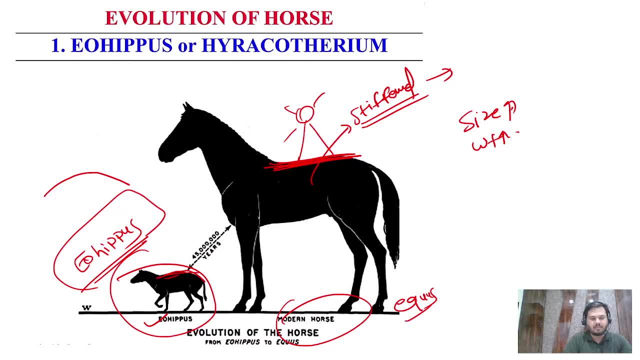 evolutionarily also it back stiffened. they were not capable of this. so actually you can see it is just a pig-like creature, or you can say it is in fox-like creature, or you can say it is in fox-like creature, or you can say it is in fox-like creature. 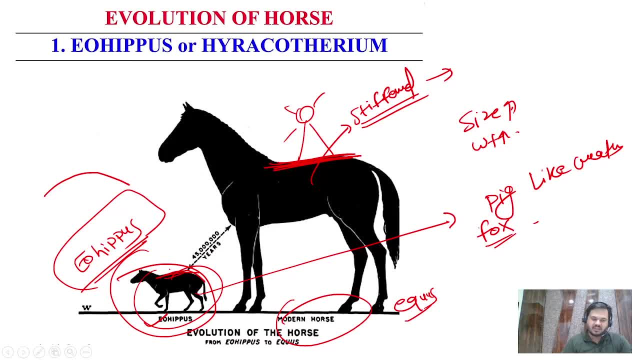 right. so size wise it was pretty much like a fox, and with time what happens is his its size of the limbs increases. now you can also see these legs are becoming very, very powerful. that is why it could you know it could do gallop, canter, all these things, like horse can walk, or then, if it is, jogging, 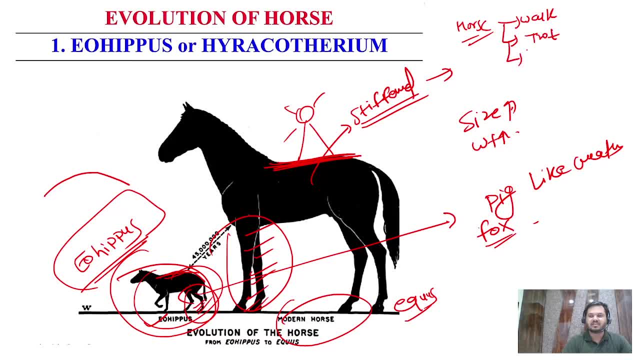 we call it trot. when horse is, you know, running fast, we call it canter, and then, when it is running fastest, we call it galloping. you must have read all this in as an english words, right, it has nothing to do with geology, but it is just for your general factoid thing, so like if you are. 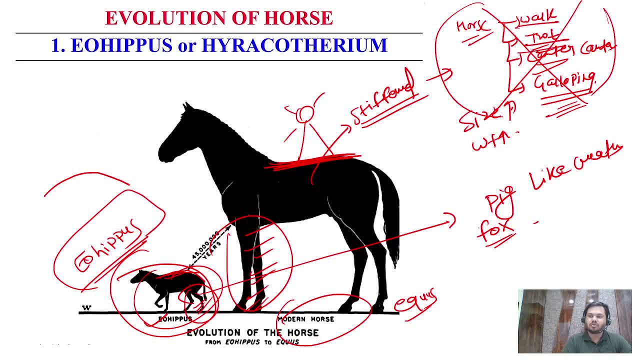 into horse riding. they will start with walk, then they will ask you to trot that horse, then canter, and if you become a pro, then you will someday gallop the horse right. so this is it. so this is what i want to discuss here, right? what are the evolutionary? 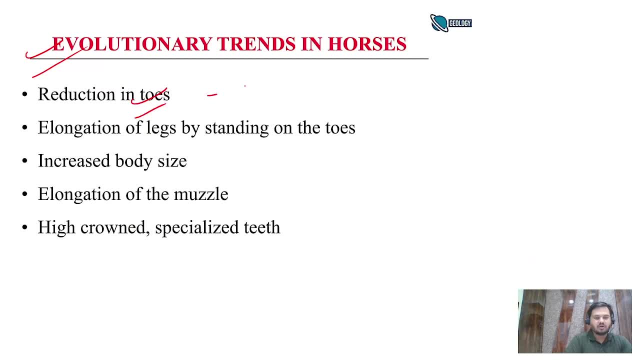 changes taking place. one is in the reduction of toes, all right, from five toe to one toe. can anybody tell me? if somebody tell me this answer, i will give him a chocolate, or give her a chocolate- all right, a big dairy milk. see why this number of toe might be decreasing. 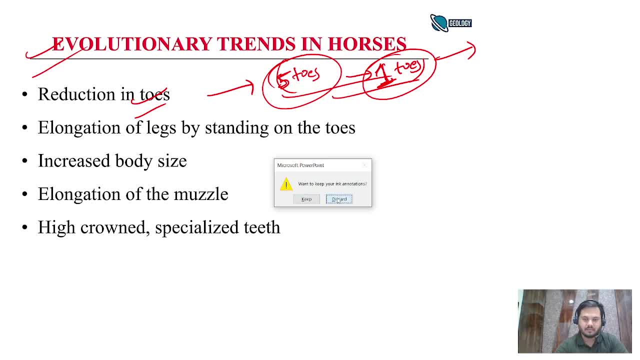 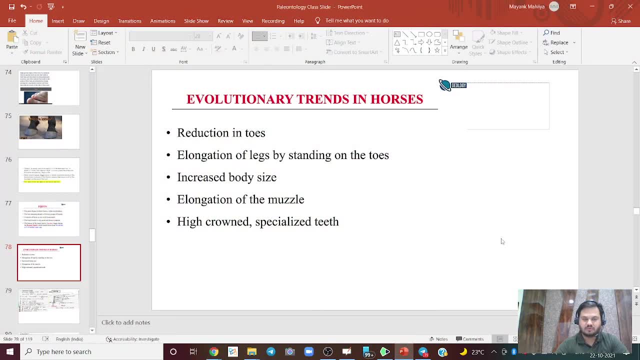 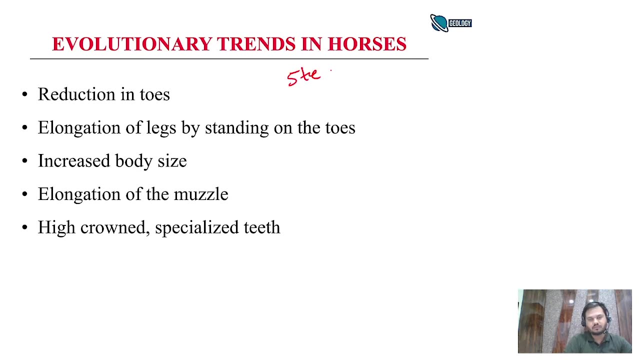 i hope you are still there, away away. yes, sir. okay, so tell me- this is a chocolate question- why there could be a decline in the toe, sir, because horse, uh, run fast just because of that reason. yeah, pretty, pretty close actually. this is the reason with one toe, like earlier. 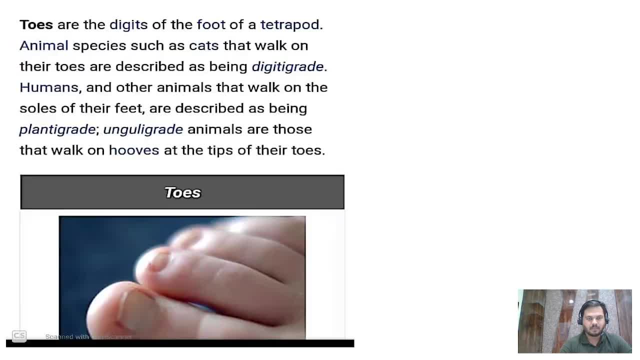 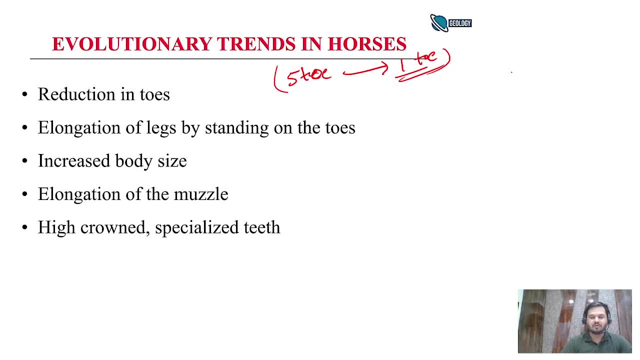 and so because planes were getting developed in north america. yes, this is very good. so it is related to both the things. what like both of you? one told that about the running- it could run fast- and one told about the environment. so actually what was happening was when your hippos originated. 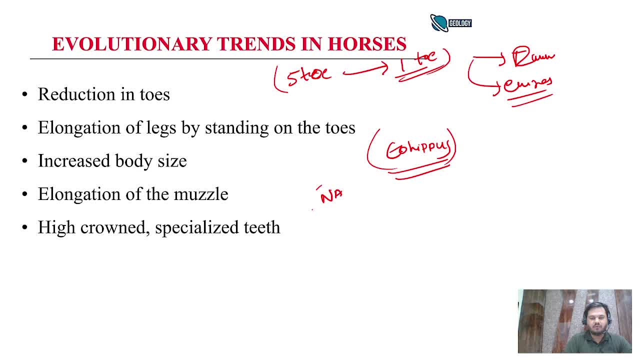 it came into existence, the climate in north america was forested. right, it was dense forest, so it is very easy to hide in the forest. you can hide behind a bush- all right, also in forest. actually, we call lion as the king of jungle. all right, the king of the forest, but actually tiger and lion, actually lion, it does. 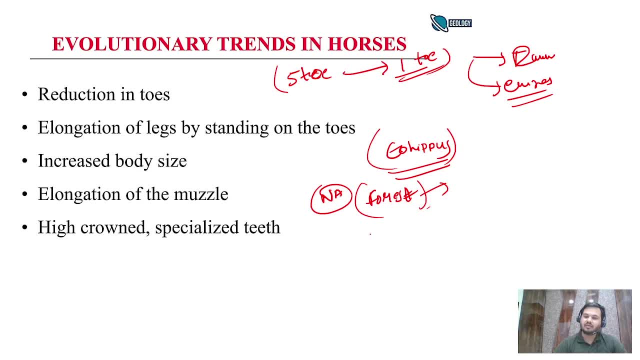 not live in forest. all right, it does not live in forest, they mostly live in grasslands. this is a very basic understanding. actually, they live in grassland because in forest- actually in dense forest- tiger can live. tiger can live in all difficult terrain, but lion don't like forested area. they live there might be. 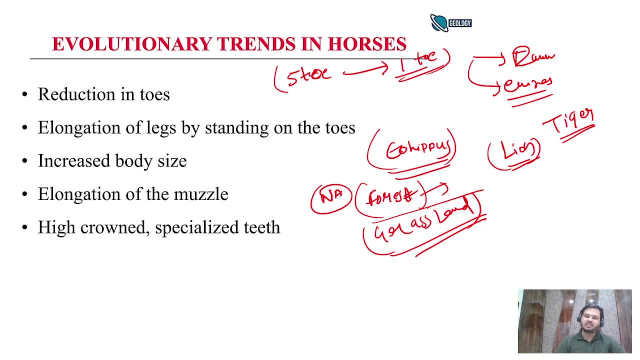 some trees, but it is essentially a grassland, all right, a deciduous forest kind of a thing. uh, so so what happens is in forest there is less room to you know, run fast, all right. so lion will be able to live in a dense forest and it will not be able to run fast because it lives in a dense. 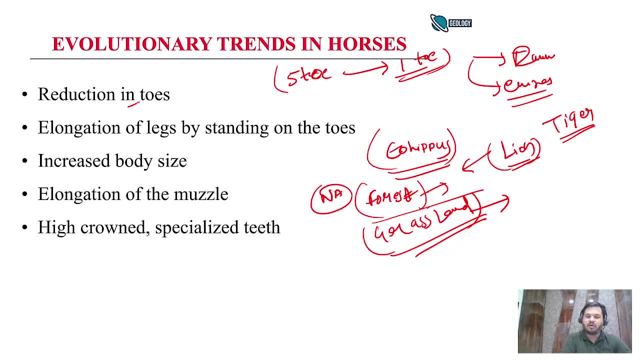 forest because it cannot hunt. in grassland it is all open. so, but but think from a point of view of horse or hot like creature. when there was forest it could hide, but when it becomes grassland it like it has nowhere to go, when if a carnivore is trying to hunt it down it has to run for its life. 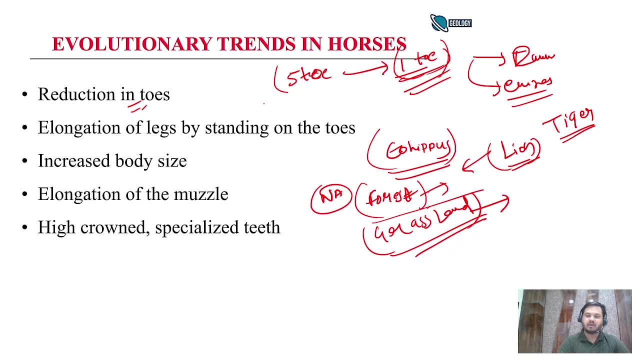 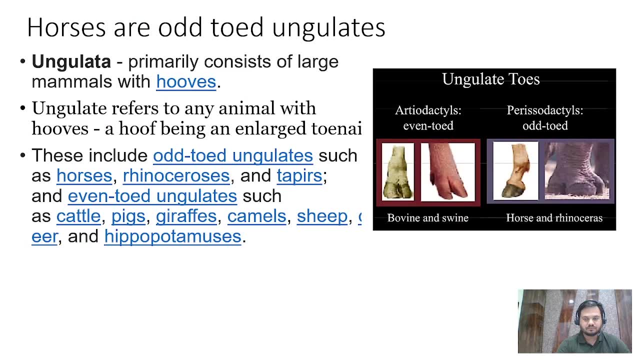 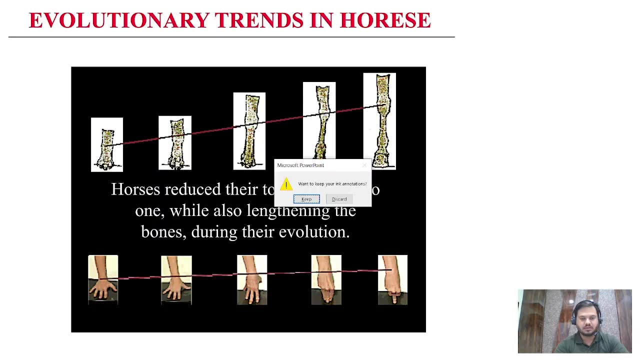 all right. so this was related to that only and it was environmental induced, but it was also for its all right. so when there are five, five all right, like there is a picture I shared, see this picture. all right, I don't know somebody is asking for one entry when we 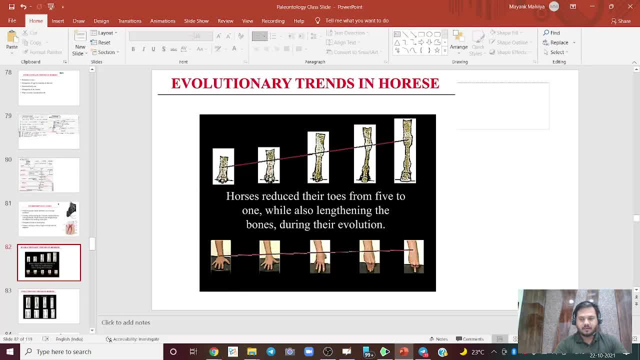 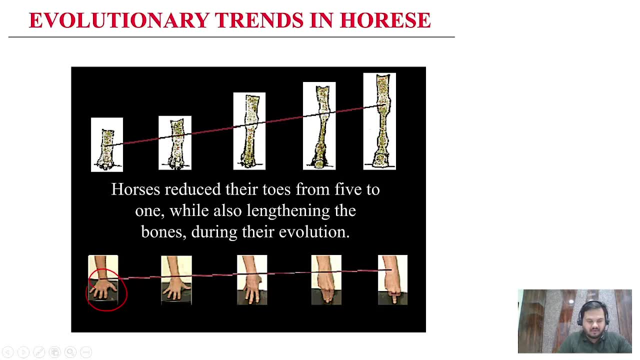 are about to end the class. all right. so see this: evolutionary trends in horse. so, if you'll see, these are five fingers, fingers like if suppose this is your foot. it is difficult to run faster, all right. similarly, see what? now it is slowly, slowly just standing on its tip of its toe. all right, on the tip of its toe. 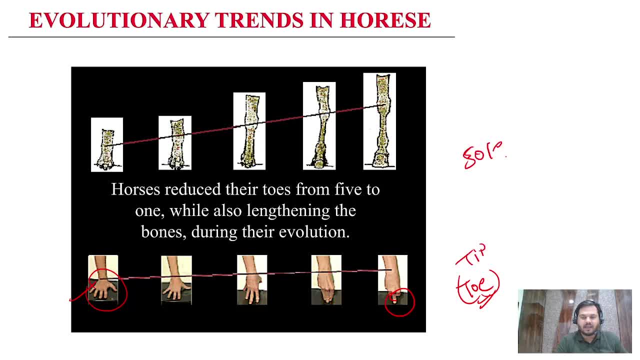 instead of standing on its sole sole, like the humans do, it is always on its on its toe, so it is pretty easy to run. all right, it is easy to run faster with this something. so this is a very, very, you know, primitive explanation audit, but this is the feel of it. right, it could run faster with one. 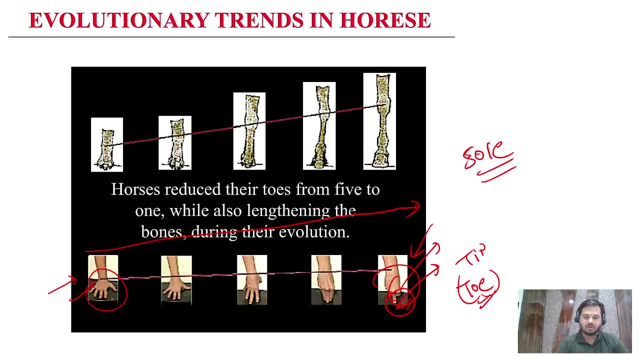 single toe, so present hearts are the single toe because of this thing only. so you can see what are the changes, evolutionary changes happening. in its lag from three or five road, the ideas key, the fingers are getting lost. they got extinct here and it is single toad so that it can run fast. another thing in 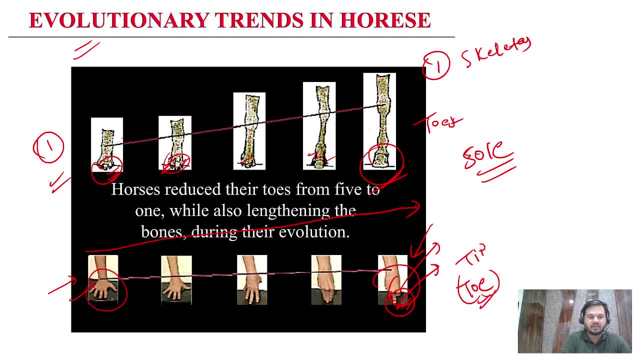 terms of skeletal, and this is a smaller bone. the bone is getting bigger and, more importantly, stronger. there are some couple of bones- a famous bonus fibula, all right, some other, so these are fusing now. here they were different, here they are fusing. so the lag is becoming. 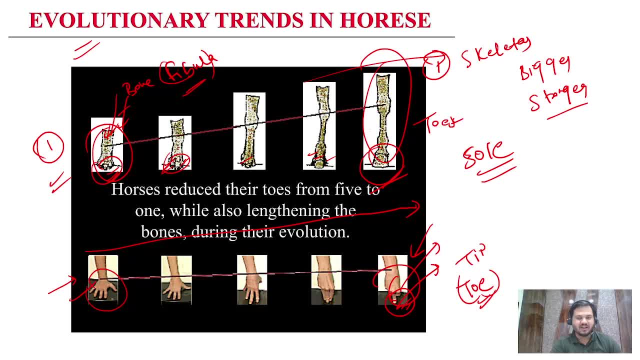 more muscular, like if you have heard about a horse hitting a kick to any person now he might even die- because these are very, very powerful legs. right, they could generate a lot of face while running and they can even fracture your multiple balls with just a single kick. so they are very, very muscular and 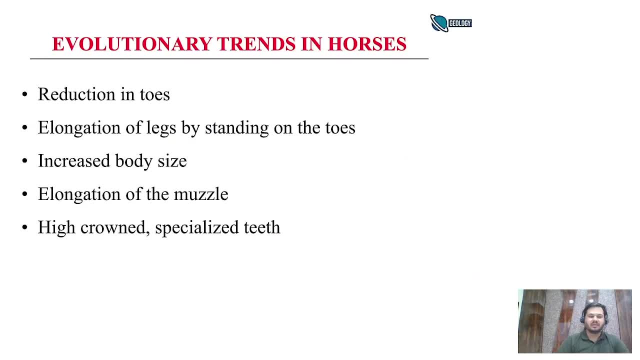 powerful legs, right. so what I'll see staging one is reduction in the toes. we dwell on the reason of it. second thing is elongation of the legs. all right, just, we saw it increase in the body size from Fox like to modern horse. all right, elongation of the muscle. 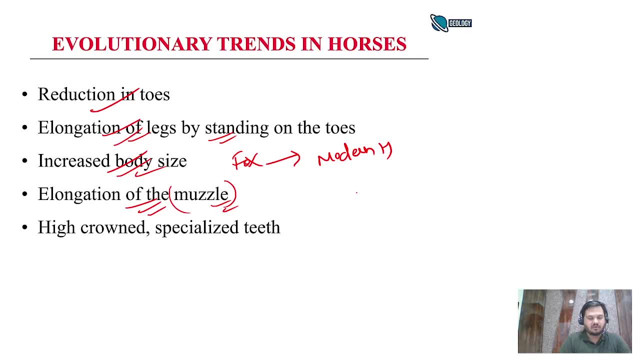 so like, what is that muscle is like, how do this? is this, forgive me for the mouth part? yes, yes, the mouth part, all right. so this is the area in front of the eyes, all right, I should be area in front of eyes, right. so this is elongation of 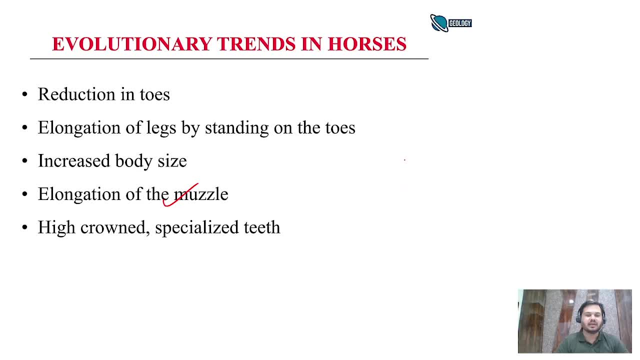 mother lappette. so this happens because it gives it could eat. it could eat the could eat grass from a distance, all right, and it even it could see. if the mouth is very close to eyes now, while eating, it becomes more prone to predation. right then there was changes in the 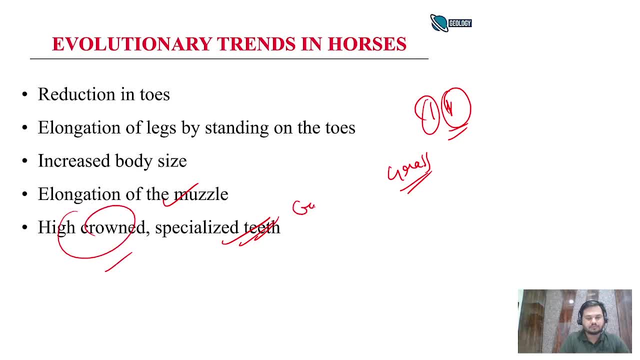 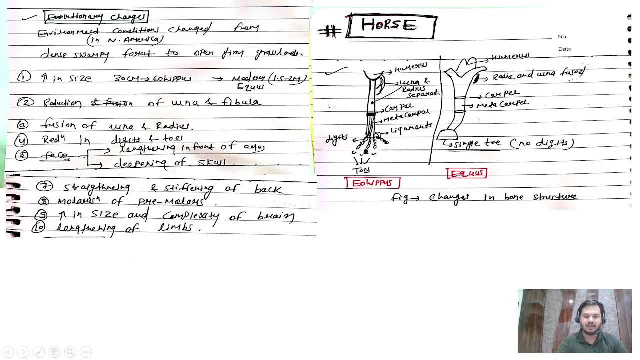 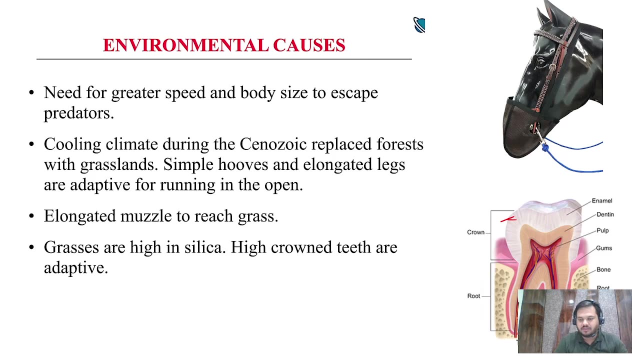 teeth right. the teeth become highly crowned like this. you need to rectify, but just these. so like what is the crown? this is a teeth, this is a human or any, any teeth of any animal. this is anatomy of a tooth. so the hard part, we call it crown. 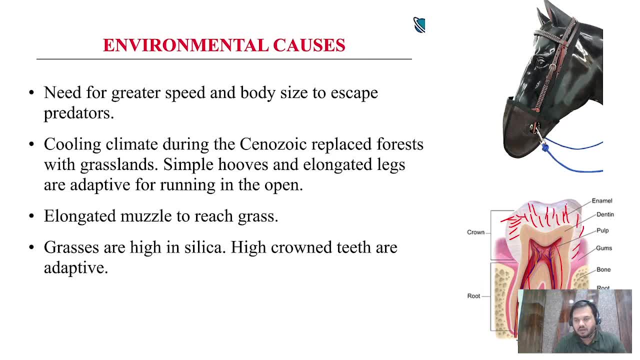 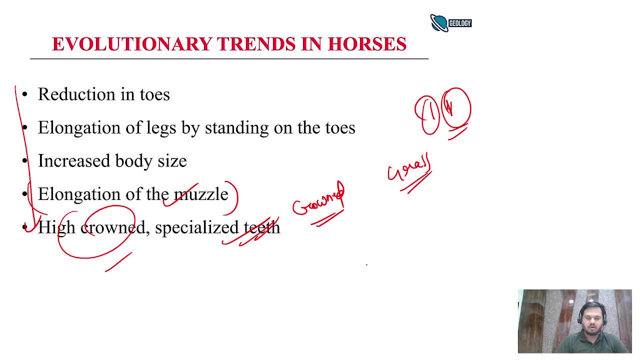 all right, this is the inner part, this is the outer part. right, crown. so this hard part is crown. so with time, as it started eating more and more, uh, grasses, and grass is like pretty hard, actually pretty hard because it has high amount of silica, right? so when it so just for protection purpose. 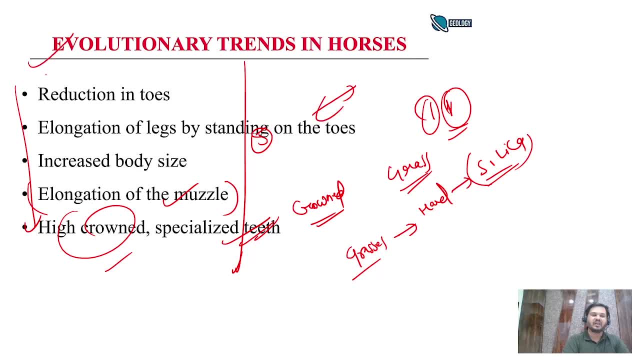 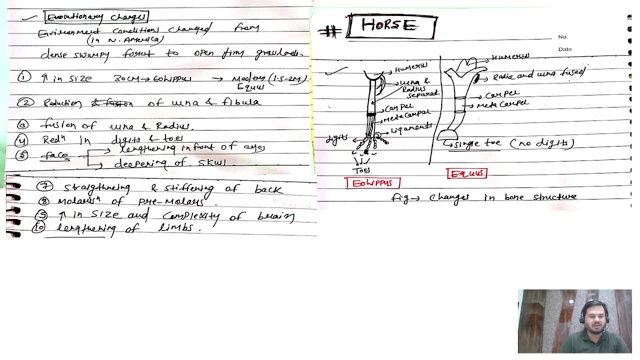 even if you are able to write this five and some general point on evolution of trend, you you have scored already 50 marks, all right, just by general understanding. so these are my bad handwriting handwritten notes. so, like i think now you will, you can understand degrees in the. 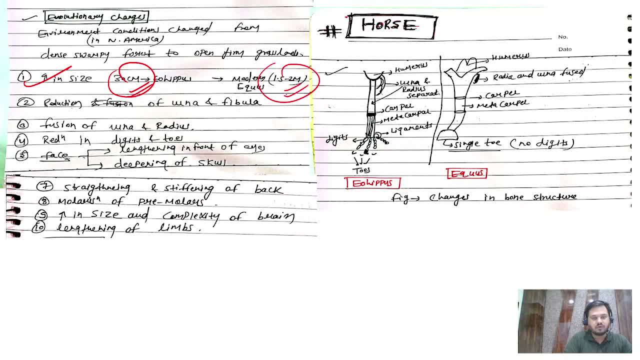 size from 30 centimeter to 1.5 to 2 meters. modern horn- sorry then, there is reduction of i, i- i use this technical term- ulna and fibula, so these are nothing, but these are the names of bones of the legs and these are general terms. if you have read science in eighth and i standard, you must be. 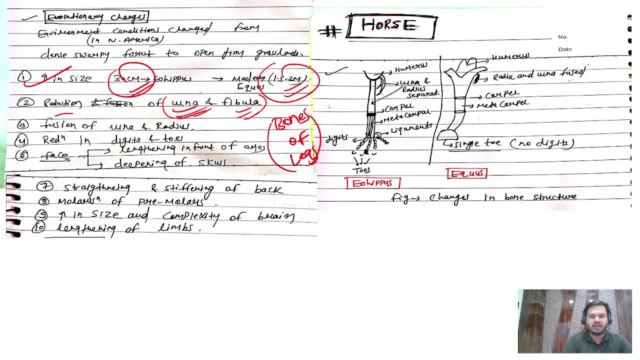 knowing all right. so actually these ulna and tubular, these are two different uh bones here. you know, this is nothing but uh lag, like yesterday somebody was asking: can i draw a diagram? right? so if you want to draw a diagram of lag, you can draw this diagram. 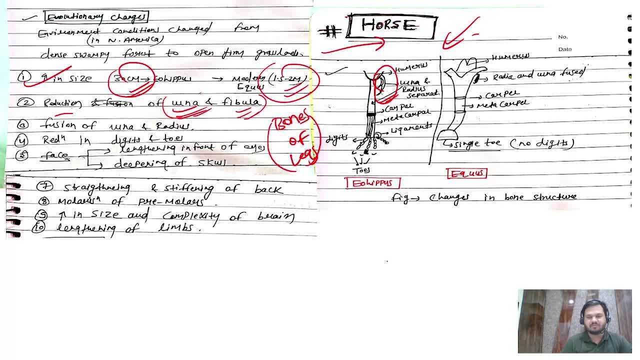 it is given in all the books and you know, everybody, like i, was pretty afraid of drawing this because i thought it will give you additional two marks, right? so this is not. you just have to draw simple legs. draw this junction. it is known as carpal. this lower part is: 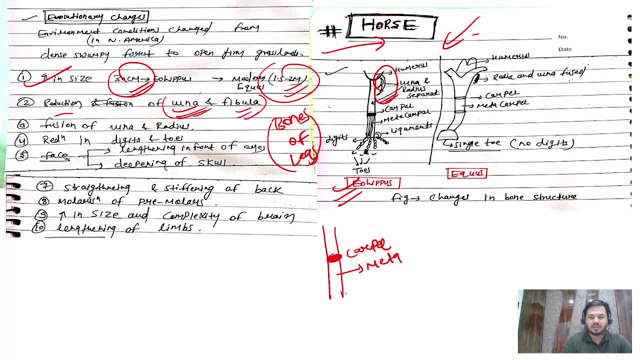 metacarpal, this is what we are talking about, your hippos. and then it has what? four, four toes? all right, something like this. so these are toes. you can draw this and not not bigger deal. they are are obviously some ligaments, and then there were some specialized bones here. all right, one is known. 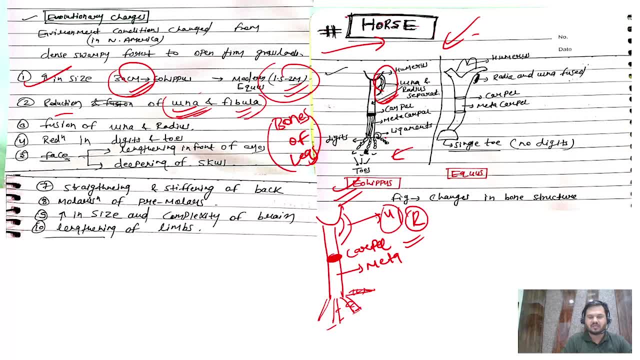 as ulna, other one is known as fibula or sometimes also radia. so what happens is this was your hip in equals. what happens is these five toes disappeared and they become. it became a single toe, all right. and also there was simplification of these. there were, like this, radia and ulna. these 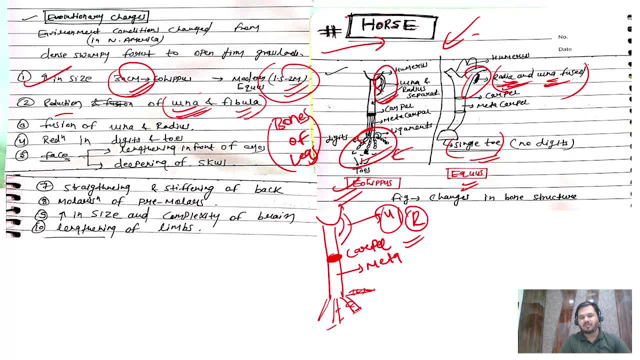 two bones. these are names of the bone, right? the somebody, somebody's, vijay, somebody's, vinny, somebody's like. these are the name of the bones. all right, so this is radia and ulna. they fuse together. so just simple diagram. you can draw nothing fancy about it, right? so, apart from this, 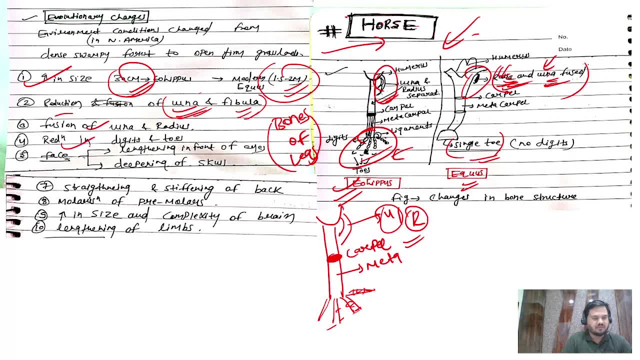 there is fusion of ulna and radia, then there is reduction in the toes. we discuss about it. what are the changes in the face? there is lengthening of the muscle or lengthening of the area in front of the eyes and there was deepening of the skull. 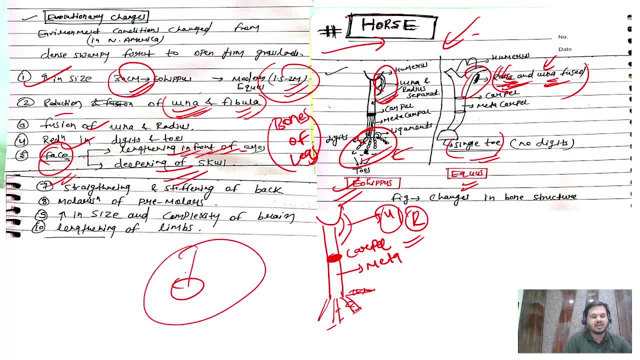 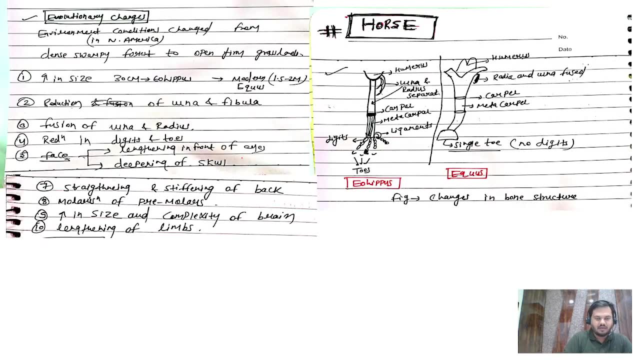 right the skull. it started to sit more deep, so it could even avoid injuries and all these things. apart from that, there is strengthening and stiffening of the back so that it could be set upon by humans in their marriages, right. so this is an evolutionary change straight. 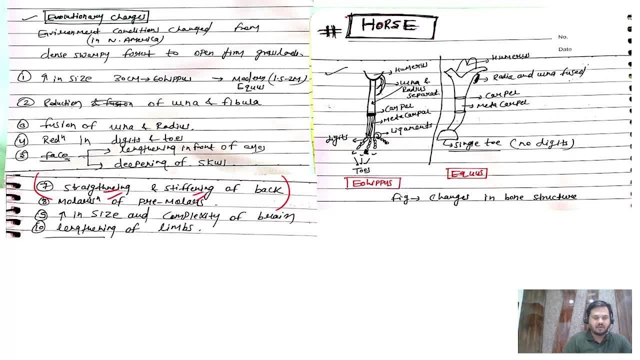 strengthening and straightening and stiffening of the back. then there was changes in some dental structure. a molarization of premolars increase. obviously this is a common for all the animals, right? what? increase in the size and the complexity of the brain, the cranial capacity increase, the lengthening of the length, all these things just by your common. 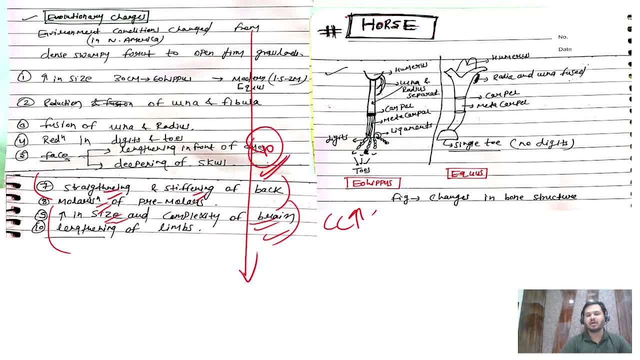 sense, you can generate these standpoints. you don't have to mug up, mug all these things right, even if you sleep today, just when you sleep, just remember, can you produce these standpoints for evolutionary changes in the horse and like. so? what does premolar means? like i? i'll cover this tomorrow and tomorrow. 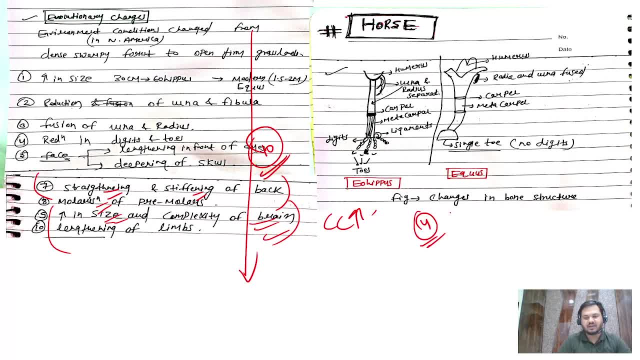 class, like the vina, we have, i think, four kind of teeth. it is about teeth. read something about it. one kind of teeth is canine and just some of the penne, penne, penne from the one we cut. we call it canine. then we have incisor now, if i'm right, anybody can help me here. the third one is: 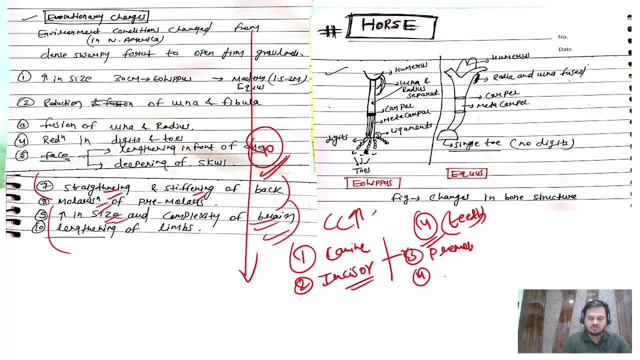 premolar. and the fourth one, the, we call it dar. right, it is molar. so if you have a man, you have a man who has the bra and you have to do the teeth. but when you have the teeth, uh, the canine has the teeth, the canine uses them. and these four 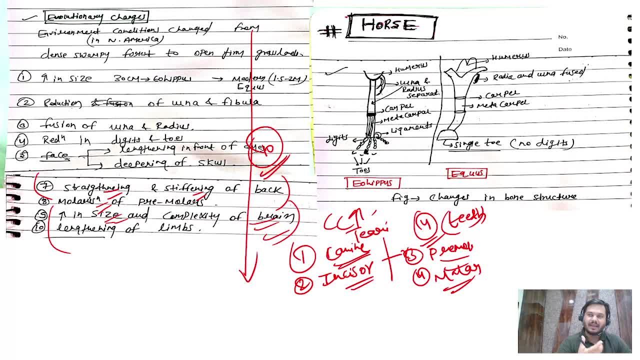 kind of teeth? uh, they have their specific purpose. the canine is used for tearing, right, if you've seen a dog, or maybe if you've seen a tiger, the teeth which are in the in front, not those the very- uh, what we call it very- pointed teeth. we call them canine and incisor: the inner. 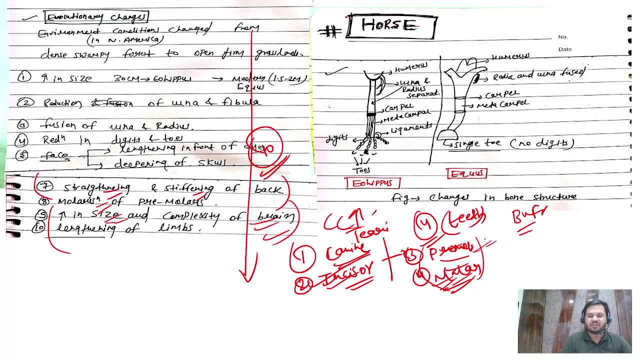 in buffaloes they have a weaker molars than a premolar. so what they do is what? they just tear the foot and they just gulp it inside and then later they digest it. so it is these. these teeths are chewers. now you chew whatever you eat. you just observe it how you eat. eat today's dinner. 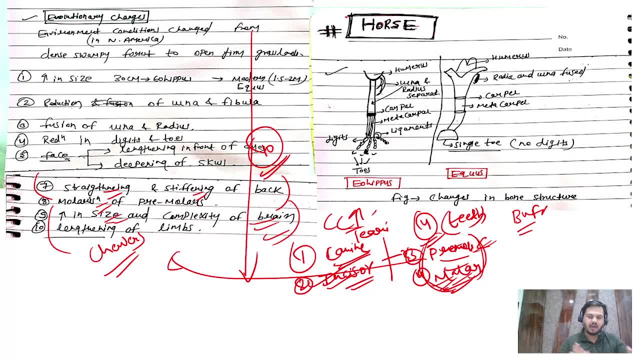 so you will eat and then the foot will go a bit deeper and you'll chew from your molars and the premolar, all right, so something like that, molarization of premolar more. i'll take up it in the next class, maybe something about dental, but i think you now know about this term, right. 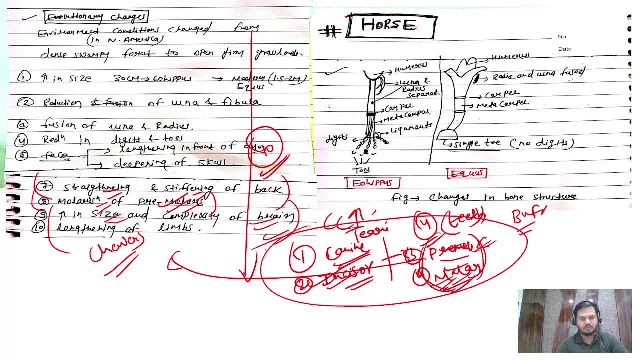 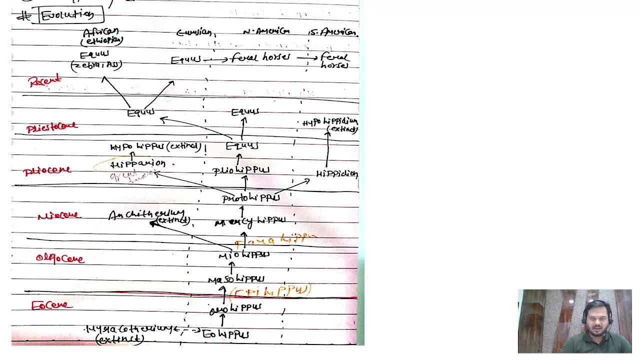 premolar and molar. this is a kind of teeth right. so, uh, this is the evolution. so, like i i said again, this is the final slide. we'll come back to it now again, i just want to tell you this slide so that when we come last it won't be. 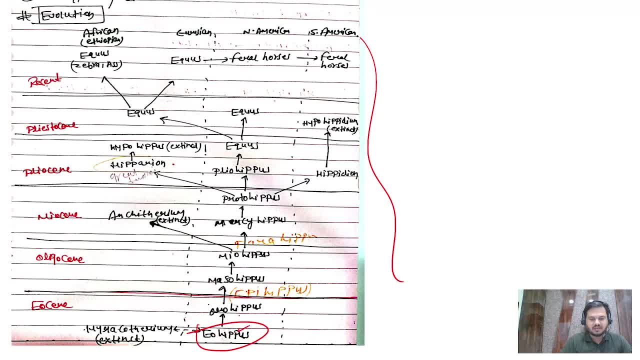 something new to you, right? so first is eohippus, then orohippus, then chemisohippus, myohippus, e, o, m, p, m, p, and from protohippus in the myosin time, now there becomes a lot of branch. one is this hippidian and hypohippidian. both of them are extinct. what hippidian, this hippidian? 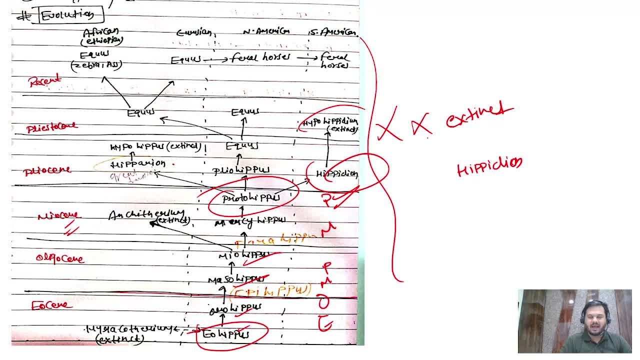 like i, i put these my notes. additionally, just to give an idea of how your own notes will be right. i could skip this. like lawrence also uses only this slide, i could also do that, but i just use these slides to give you an idea. but unfortunately i don't have a very good handwriting so it hinders a bit. 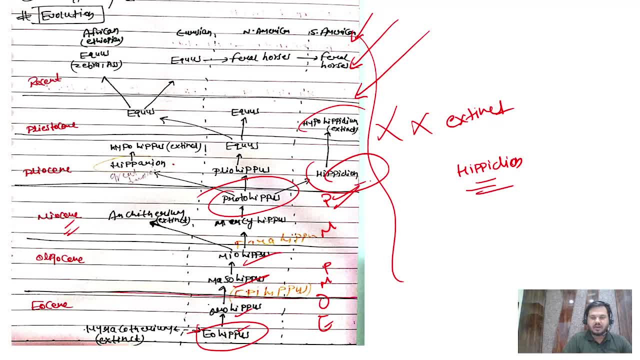 of learning. but don't worry, i'll write it here like: this is hippidian, this is hypohippidian. from protohippus there come this plyohippus and some variety of equus which got extinct. and right there was this very famous hipparion, also right, hypohippus, it got extinct. and then from this: 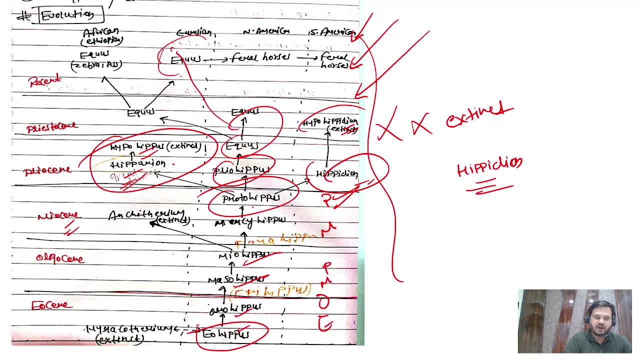 equus, we have this modern horses, these modern horses converted into feral horses and something like this right and from here, only this equals only if we have other cousins of the horse. what are the cousins of horse? this zebra? all right, these are the cousins of horses, these are zebra. 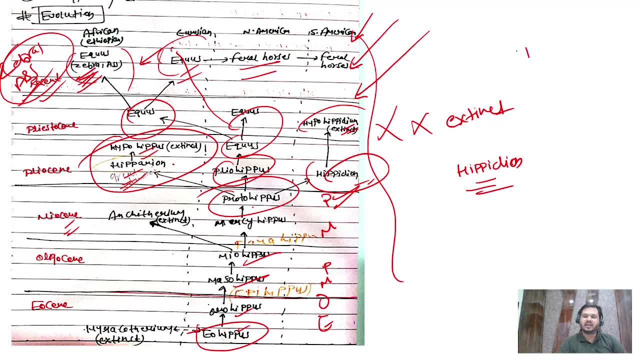 where do you find zebra? can do you find zebra in india? they are finding africa only. you must have seen in documentaries in very, very, very favorite prey of a tiger and maybe cheetah, and they always hunt these jabras. so these are so something like this, similarly all right. one. one again thing we should remember is: 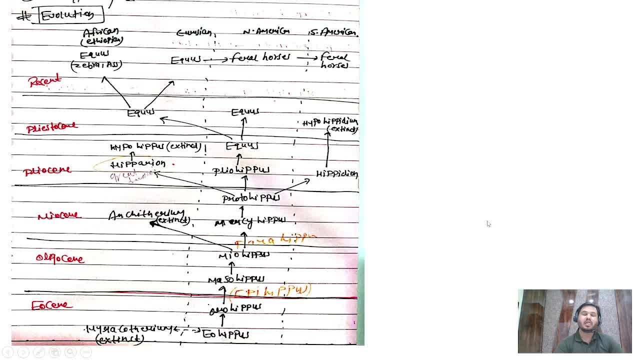 unfortunately, even though the north america is the cradle of human, sorry cradle of horse evolution. but presently, like few years ago, few like i will tell the time in the slide- horse got completely extinct from north america, right, even though horse evolved in north america. so like this is the 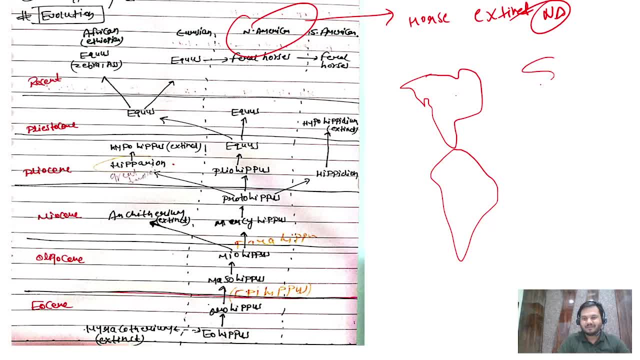 what is this? can anybody tell me? what is this? what is this? okay, so this is north, this is europe. this is north america, this is south america, this is atlantic ocean, this is pacific ocean. right, like see, i draw, i admit like i am using it. 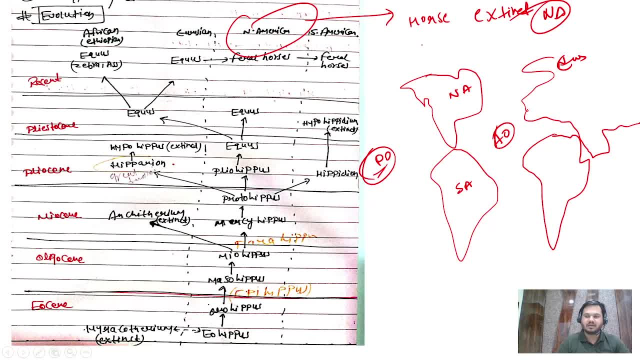 a pen tab, so that is why it is not coming very neat. but i like, like me, you should also be able to draw the diagram of world map in 20 seconds, right, so practice this. that this comes very handy in. generally, i think plays really good. this is a very important slide. jeff Тиш coalition. thank you. 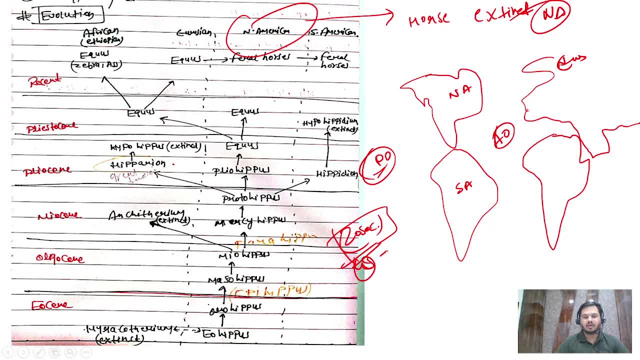 general studies, paper one, paper three, even in two international relations. this is very, very handy, even in geology it gives you one mark extra. all right, so draw it in 10, 20, 20 second. i will. in next class i will draw it in a more later way. so they, even though they originated here, then with 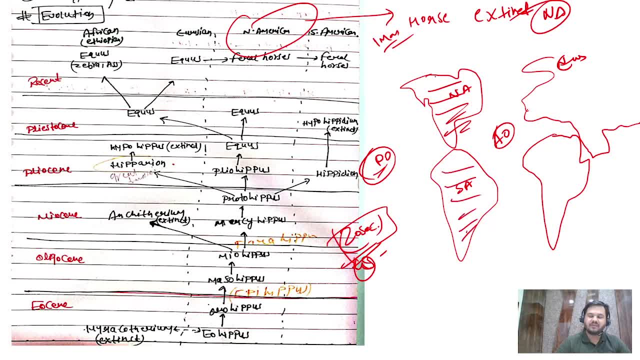 time they, you know, they are found here also. and when? what happens was then, when there was ice ages. i say here, this is alaska and you must have heard about bearing state, right, so there is a bridge, bearing bridge, we call it so- when there was ice age. in ice age, what happens to sea level? 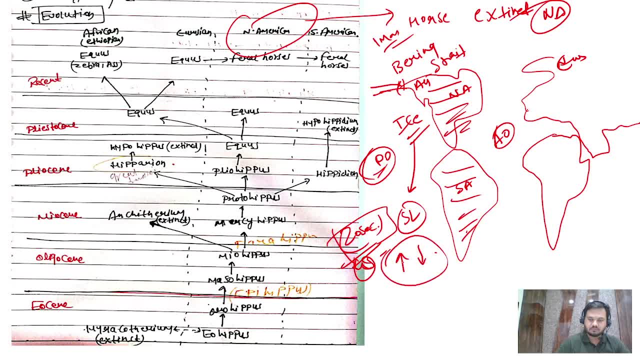 it increase or decrease? yes, it decreased, so sea level go much down and you know this. rocks got exposed, so we call it a bearing bearing state bridge. so what happens is this: north america, alaska, got connected to russia, siberia, through this bridge, so these horse migrated to here, they migrated to siberia, eurasia, basically they. 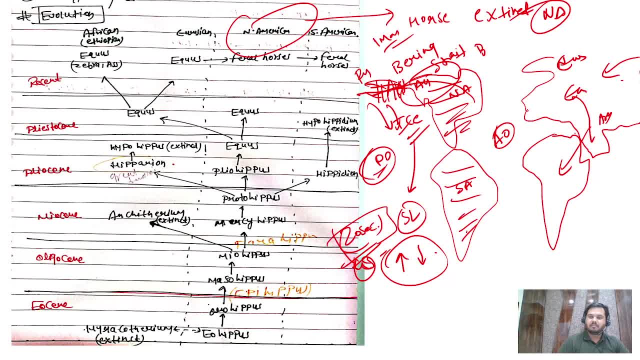 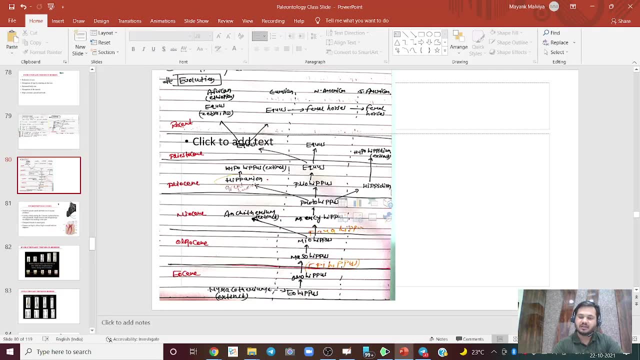 migrated to arab right africa, everywhere, but unfortunately, due to whatever reason which is yet not certain, they got wiped out from americas. right, they got wiped out from americas, so horses are not naturally formed in americas presently. they did got, you know, reintroduced there in 16th century by 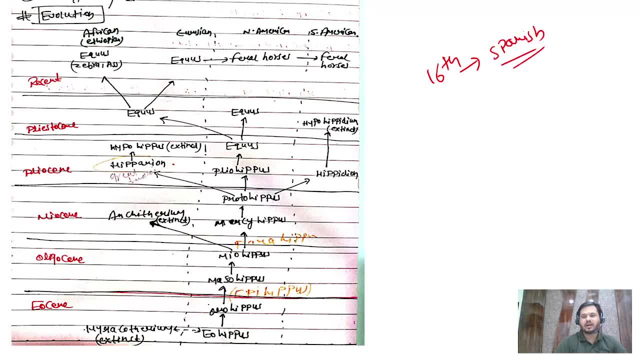 spanish people, right. so like this is something so you can see whatever was happening in north america. here is north america, eurasia, south america. i like this was a diagram in the book so i copied it here so see all this evolution was happening in north america. 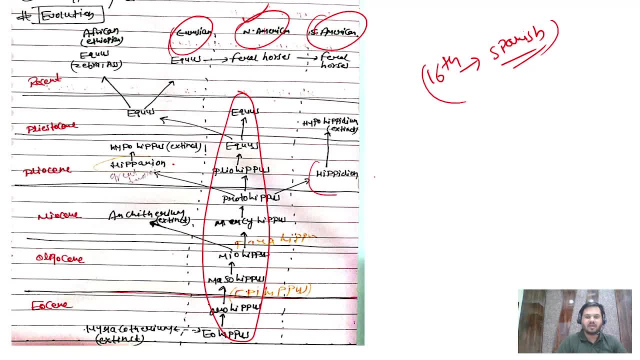 this proto hippos. it got, like, migrated to south america in hip and it converted into hippidian and then hypo hippidian and it also got extinct. here this north american equals also got extinct, right. so here this equals. it migrated into eurasia during pleistocene time like. can you see the diagram here, vijay? and 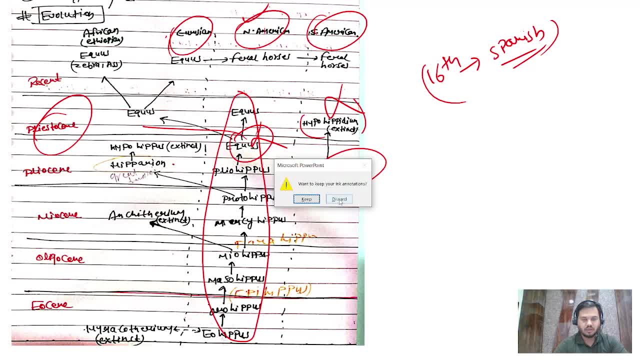 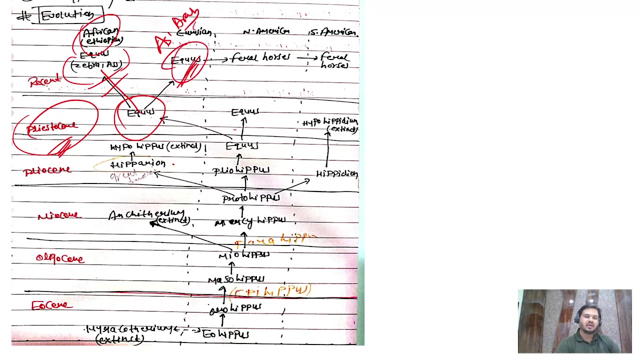 everyone: yes, okay, right. so see, this is this same species. migrated here in eurasia during the ice ages, during pre-stress in time, and then in africa it evolved into zebra and s right in, mostly in utopia. another reason: tanzania right. and when it came to af, like asia, especially arab countries, like here, it converted into equals. 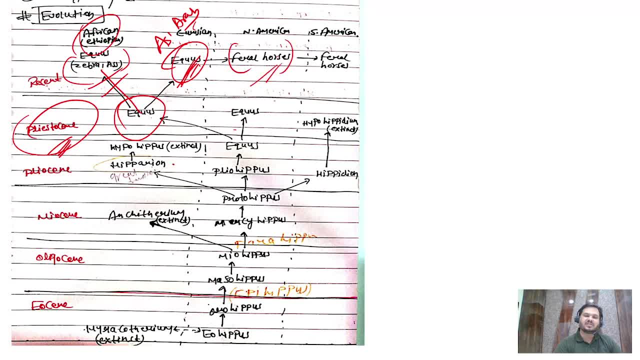 and from equals like this, uh, non-domesticated wild. we carried it to north america and similarly we carried it to south america, so it is not naturally found, it is human induced. this chain is human induced. right, you don't have to write so much in exam, but just if you like. i i shared this because 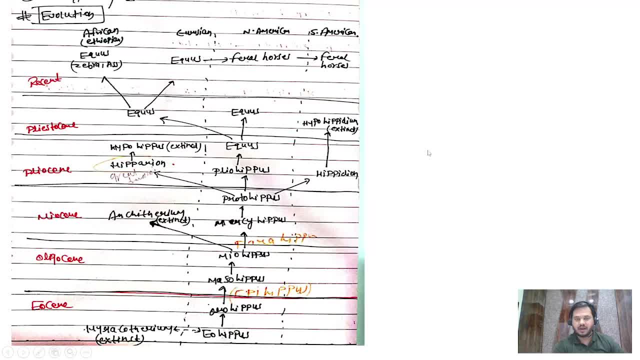 this will open up some other dimensions of your understanding, right, you don't know, but the examiner who is checking the copy knows that they have been extinct in north america. so in this diagram, just writing, just putting this dotted diagram here, i have you know, included a lot of. 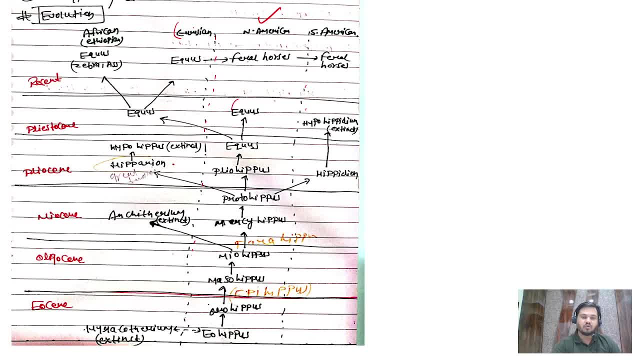 detail is there are no longer any naturally occurring horses. right, they got extinct here in itself in places in time, but some of them migrated to africa and eurasia. we have the modern horse naturally here, so, right, just using these three words and putting this dot, now i have given. 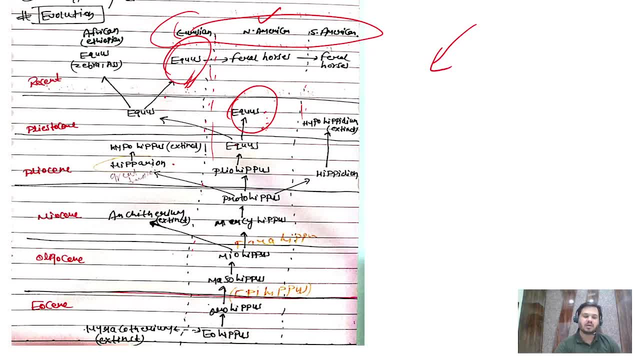 you some information which might not appear obvious to you if you are new to this topic. right, this uapus sometime is also known as hierarcho theorem. right, but i found this more fancy, more easy to remember. your hippers, right? so i think, uh, we have a decent amount of right this. 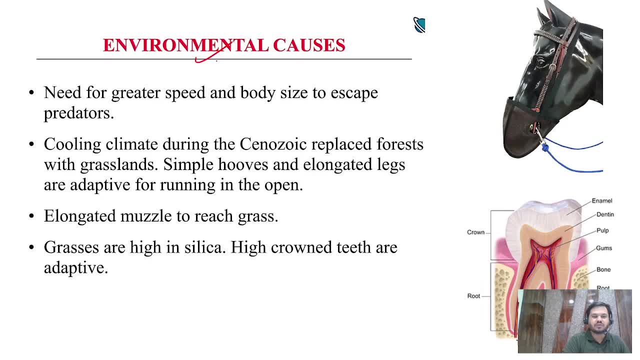 is the last slide and then we will stop right. so what are the environmental causes? leading to this? evolution is since forests say, to the grassland in cenozoic time. so there was a need for greater speed, all right. so for greater speed they also need more body size, more powerful legs to escape from predators. this was one of the 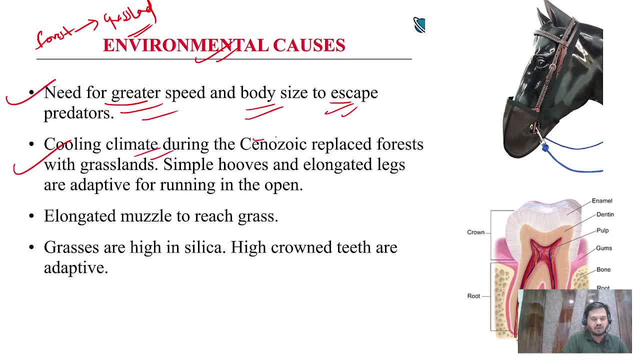 rating, all right. another thing is cooling of the climate in the cenozoic, where it induced the replacement of forest to grassland. all right, then this elongated muzzle to reach to the grass easier, all right. grasses became high in silica, so seeds become more crowned. it is an adaptive feature. so this is it. so this we discussed already. 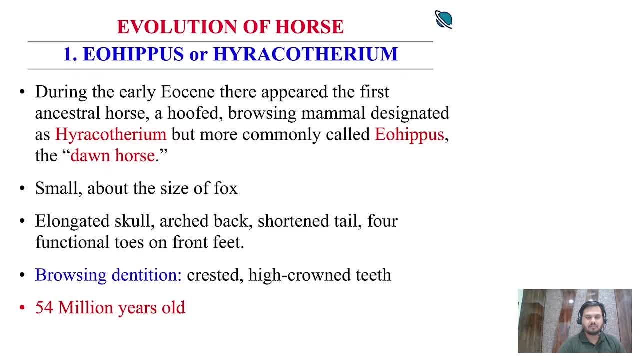 this diagram and again the same diagram in some another form. right, so like does it. that is it. we will end the session here tomorrow. we will take uh like, we will spend 15, 20 minutes and we will take up each and every like we did for human. we will dwell on all specific uh. ancestor of horse.